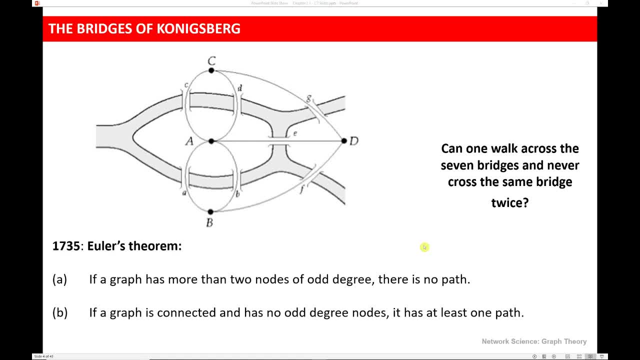 So in 1735, the property he discovered and proved was that if a graph has more than two nodes of odd degree, there is no path. As we'll talk about in this chapter, the degree of a node is how many edges are connected to that node. So what he showed was that if a graph had more than two nodes of odd, 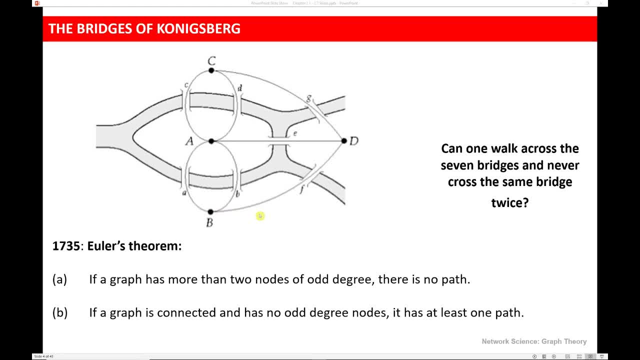 degree, meaning that they had an odd number of connections, that there wasn't a path. And we can see, looking at this graph, that that is what we have, because nodes B and C have three connections coming out of them, as well as node D. In fact, I think every single node in the graph is of odd degree. 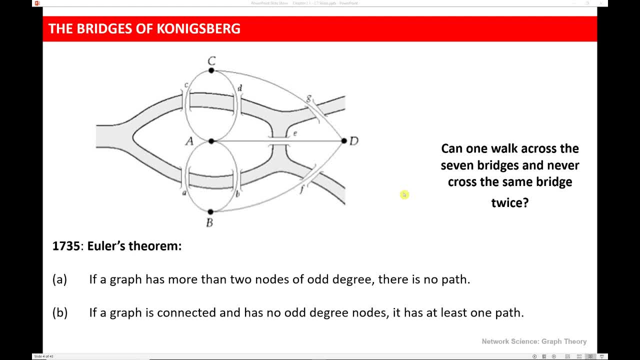 And if you try to trace over the bridges you can see that you can't really solve the problem. He also showed that if a graph is divided by two, the connective side of the node is yellowed out. So if a graph has two nodes, then it's a path, But if a graph has one node, then it's a path. 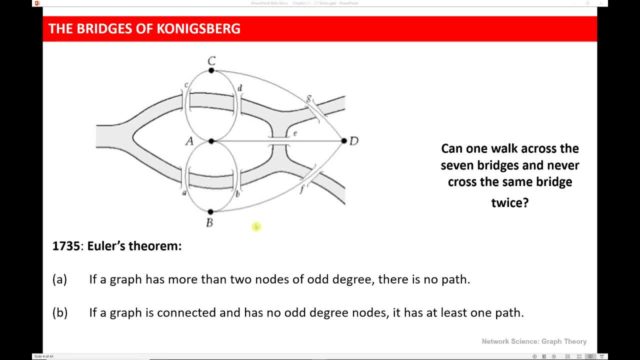 graph is connected and has no odd degree nodes, that it has at least one path. Euler's discovery is interesting to us for a couple of different reasons. First, as I said before, he showed that graphs actually have properties that are immutable. Secondly, it's interesting that he was able to 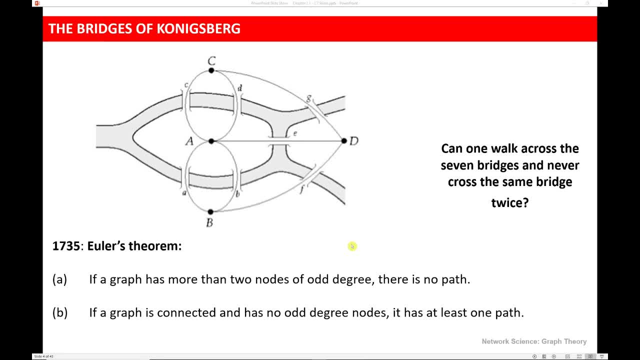 solve this problem based on modeling something in the real world, And I think that as we progress through the class, that's what you're going to see is that each graph has a story to tell based on its components. Let's define some basic terminology for talking about networks and graphs. 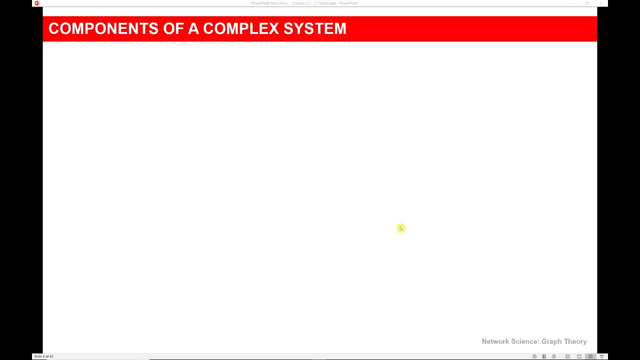 When we talk about graphs or networks, we're talking about a complex system. In this system, we have several components. First, what we have are the nodes, or vertices. I'm mostly going to use the term nodes to refer to the points in the graph. These can refer to almost anything. They 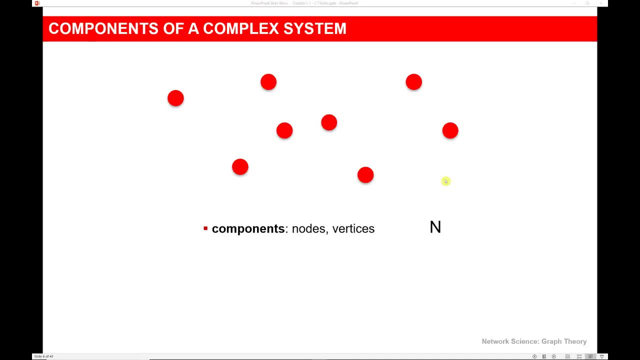 can refer to actors or criminals in a criminal network or people in a business. A capital N is going to refer to how many nodes are in the system, And then we have the nodes or vertices, And then we have the nodes or vertices, And then we have the nodes or vertices, And then we have the. 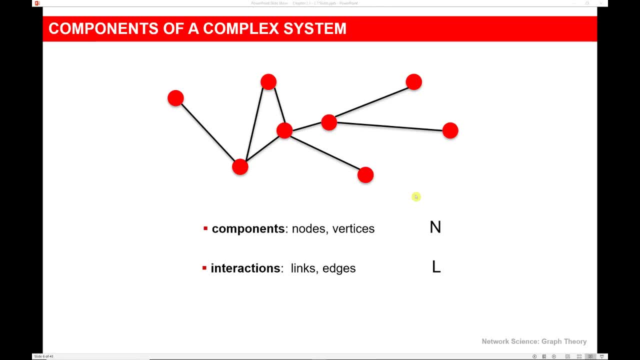 And the networks that we concern ourselves with. we will also have links or edges, And the links and edges represent the different interactions or relationships that we have among the nodes or the vertices. So this could be a connection representing that two people have acted in the same movie. 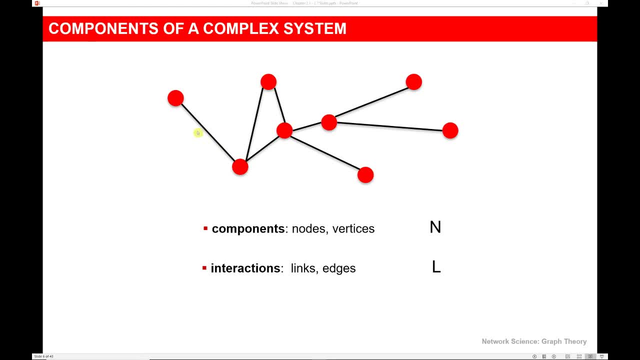 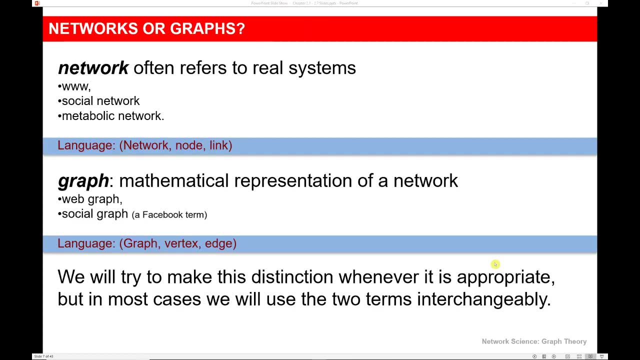 that two people have published a research paper together or that people share information at work. When we combine the nodes and the edges, we have our system or our network or our graph. There is a distinction between network and graph, although we're going 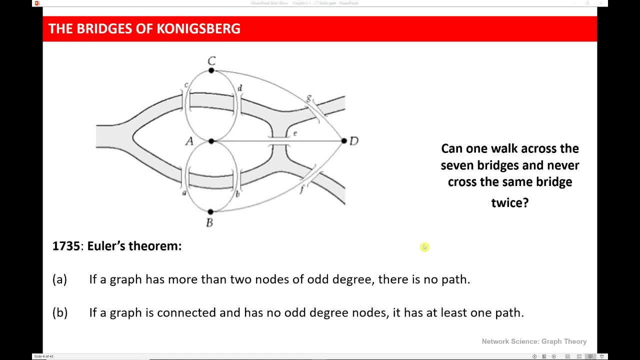 So in 1735, the property he discovered and proved was that if a graph has more than two nodes of odd degree, there is no path. As we'll talk about in this chapter, the degree of a node is how many edges are connected to that node. 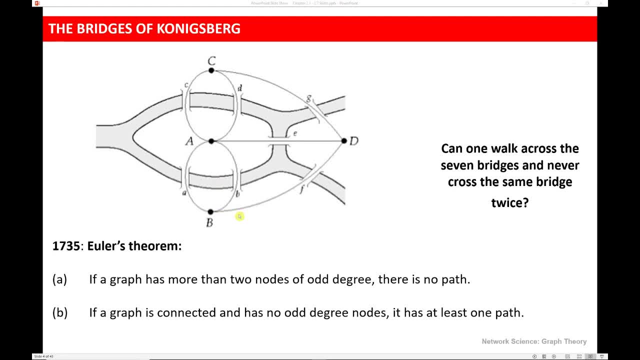 What he showed was that if a graph had more than two nodes of odd degree- meaning they had an odd number of connections- that there wasn't a path. And we can see, looking at this graph, that that is what we have, Because nodes B and C have three connections coming out of them, as well as node D. 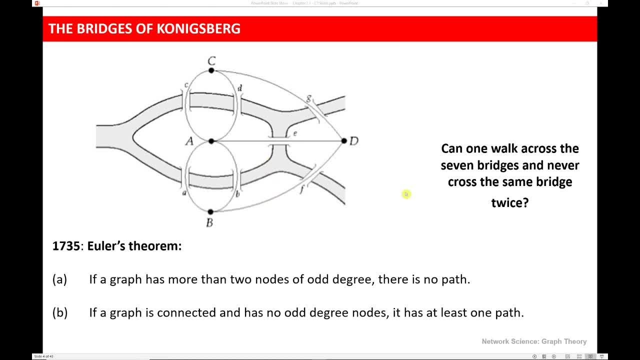 In fact, I think every single node in the graph is of odd degree. If you try to trace over the bridges, you can see that you can't really solve the problem. He also showed that if a graph was connected to a node of odd degree, there would be a path. but if there were many changes, for example, 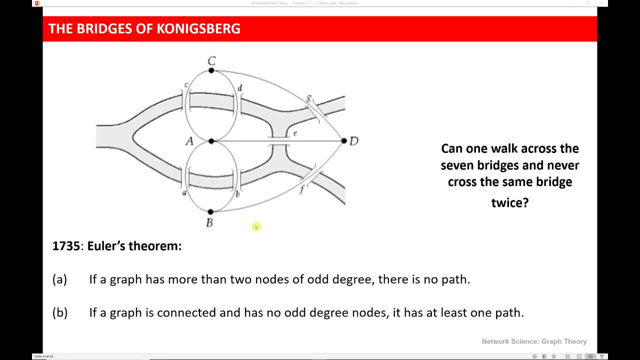 the bounds would be different, The graph would. we could easily contributing structures across the rest of the outside facade. With that in mind, we can study some space-based method. graph is connected and has no odd degree. nodes that it has at least one path: Euler's discovery. 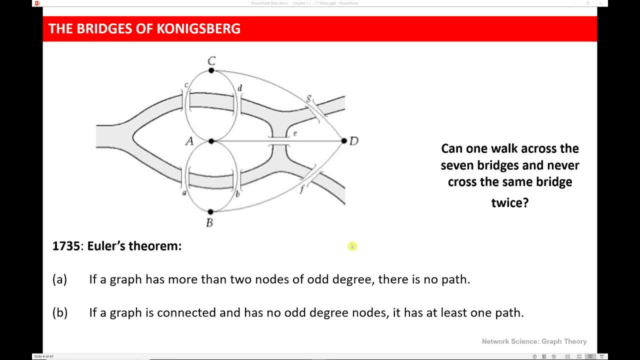 is interesting to us for a couple of different reasons. First, as I said before, he showed that graphs actually have properties that are immutable. Secondly, it's interesting that he was able to solve this problem based on modeling something in the real world, And I think that, as we progress, 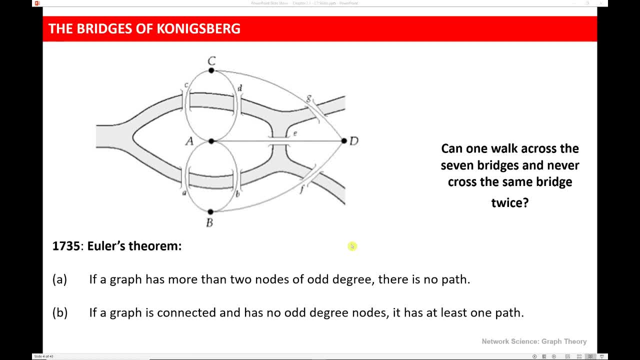 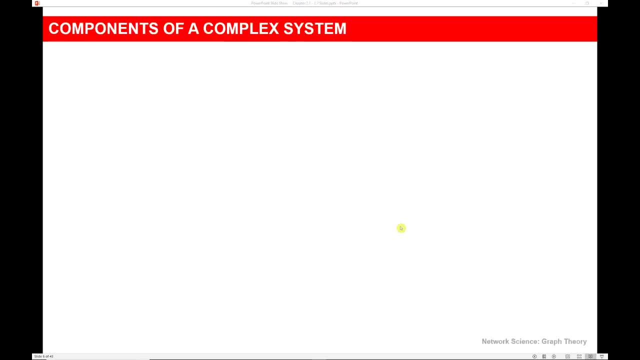 through the class. that's what you're going to see is that each graph has a story to tell based on its components. Let's define some basic terminology for talking about networks and graphs. When we talk about graphs or networks, we're talking about a complex system. In this system, 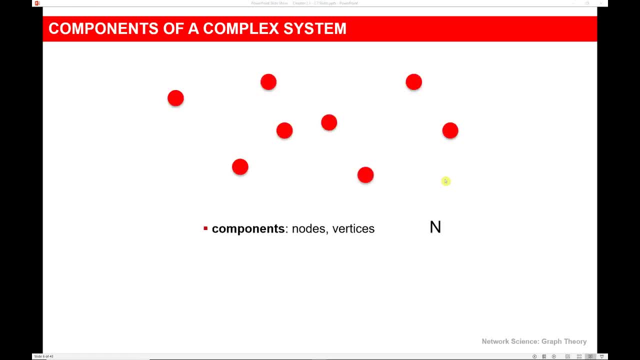 we have several components. First, what we have are the nodes or vertices. I'm mostly going to use the term nodes to refer to the points in the graph. These can refer to almost anything. They can refer to actors or criminals in a criminal network or people in a business. A capital N is 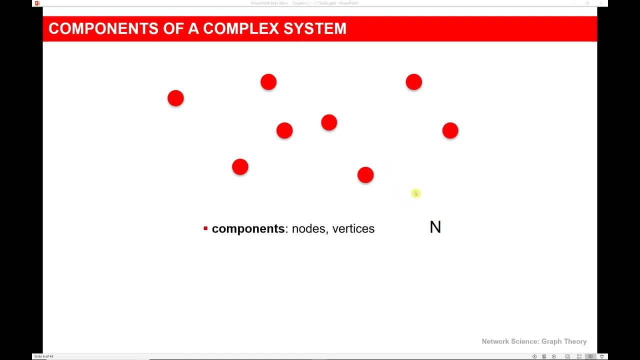 going to refer to how many nodes are in the system, And then we have the nodes or vertices, And then we have the nodes or vertices, And then we have the nodes or vertices, And then we have the And the networks that we concern ourselves with. we will also have links or edges, And the links 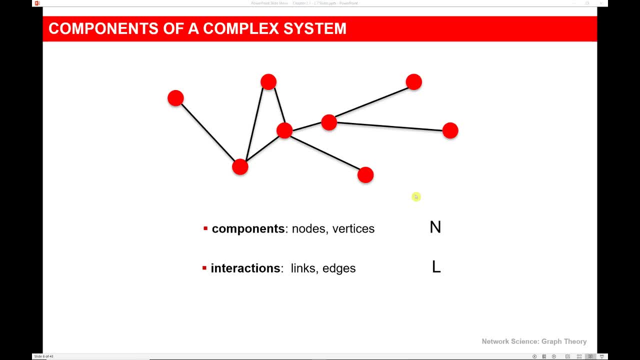 and edges represent the different interactions or relationships that we have among the nodes or the vertices. So this could be a connection representing that two people have acted in the same movie, that two people have published a research paper together or that people share information at 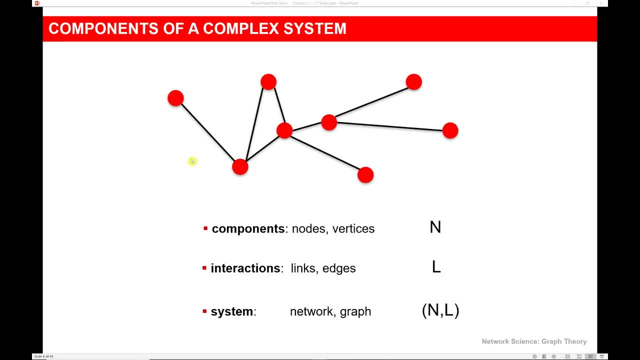 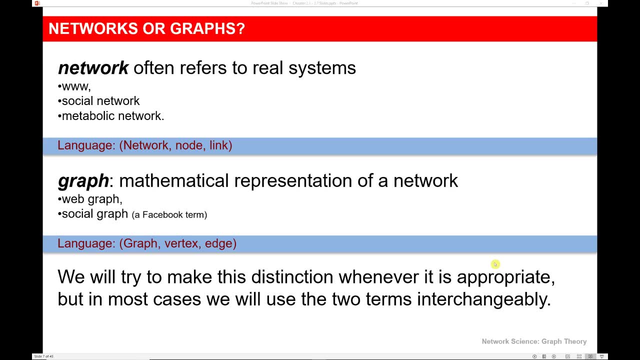 work. When we combine the nodes and the edges, we have our system or our network, or our graph. There is a distinction between network and graph, although we're going to use the terms interchangeably. A network often refers to the real system. So, for example, 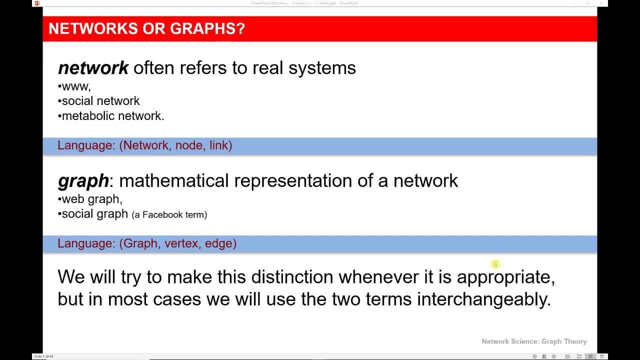 a worldwide web or a social network, or a metabolic network. When we talk about networks, we usually use the terms nodes or links, whereas a graph is a mathematical representation of a network. This could be without using labels or names for that matter, like a web graph or a social graph. 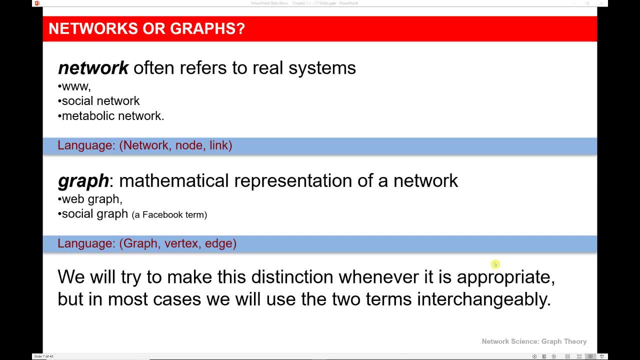 The social graph is actually the term that Facebook uses in their API for collecting data. The language you use for graphs is typically vertex and edge. So again, if we have to make this distinction, we will when it's appropriate, but in most cases we'll just use the two terms interchangeably. This is the. 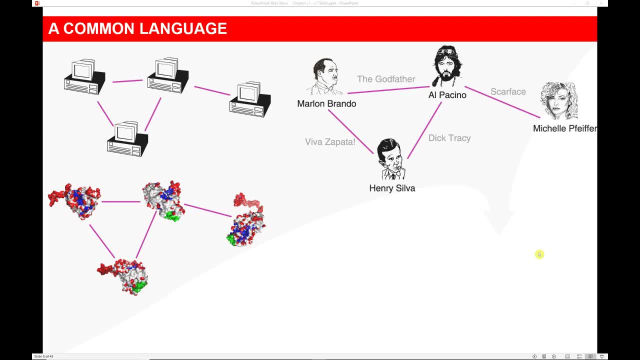 simple language that we'll use in order to describe real networks. You can see here a few different examples. This illustration shows the difference between network and graph. The underlying graph of each of these networks is actually the same. It's a graph of four different nodes and four 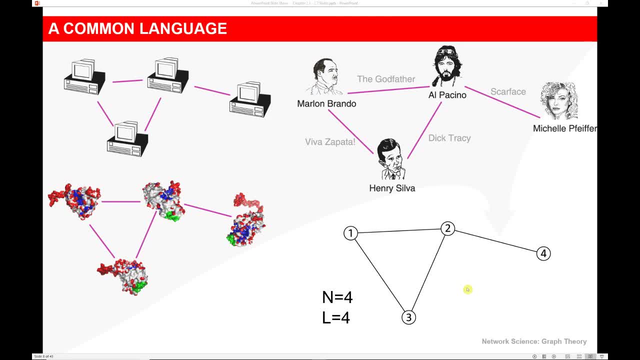 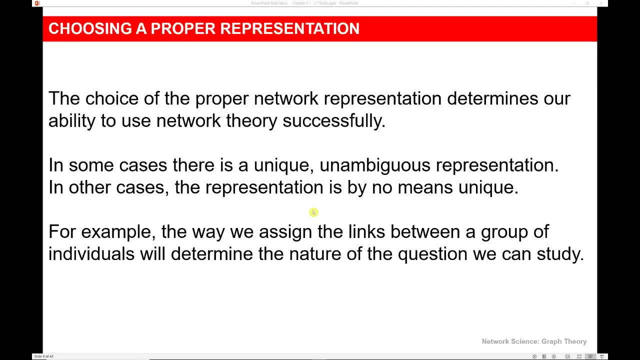 different edges or links, but we can actually overlay different real-world networks. So if we're looking at a network, we can see that each node represents a different actor and the link represents a movie in which they both acted. Choosing a network representation is very 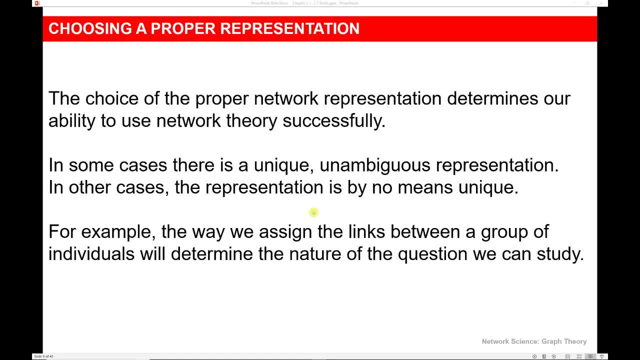 important, as the choice of the proper network representation determine our ability to use network theory successfully. In some cases there's a unique, unambiguous representation, and I think for most networks in this course that's what we'll have, But in other cases, 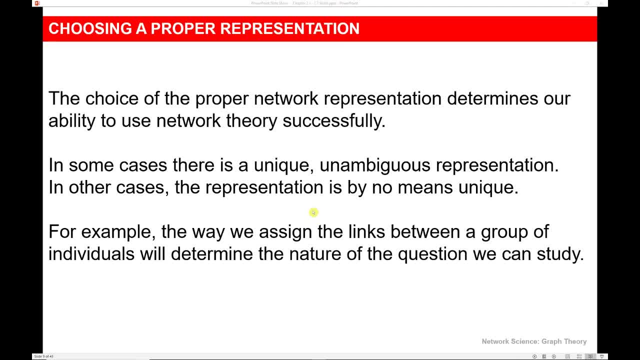 representation is by no means unique. For example, the way we assign the links between a group of individuals will determine the nature of the question that we can study. For example, I could create a network of all of the faculty in the CIDM department and I would have to decide. 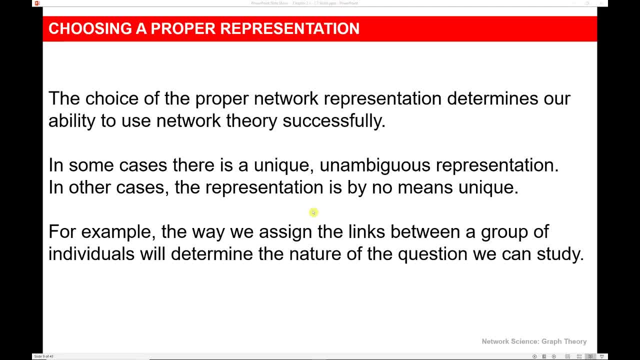 what kind of link I would want between each faculty member. Would the link represent simply that they work together, that they've taught the same course, or perhaps that they've researched together? The choice of the link would determine what kind of analysis we could do with that. 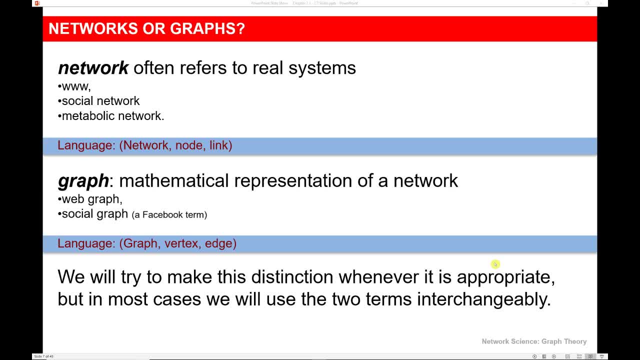 to use the terms interchangeably. A network often refers to the real system, So, for example, a worldwide web, or a social network or a metabolic network. When we talk about networks, we usually use the terms nodes or links, whereas a graph is a mathematical representation of a network. 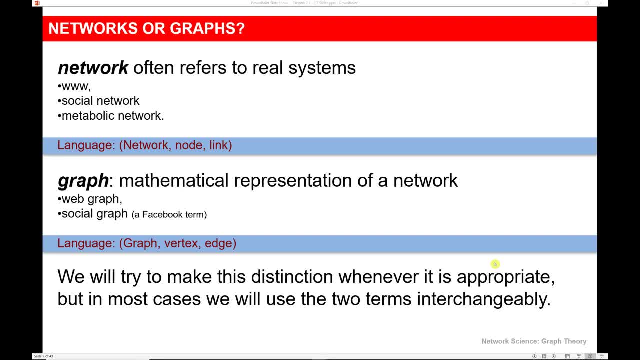 This could be without using labels or names for that matter, like a web graph or a social graph. The social graph is actually the term that Facebook uses in their API for collecting data. The language you use for graphs is typically vertex and edge, So, again, if we have to make this distinction, we will when. 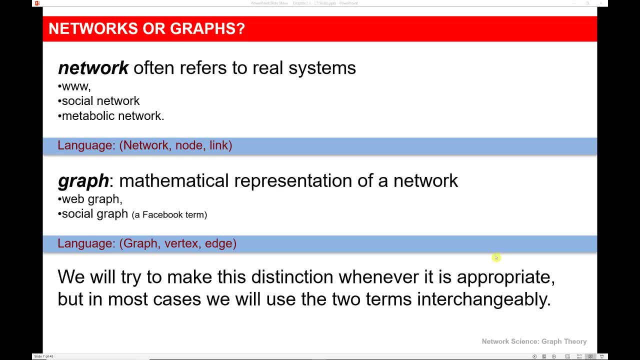 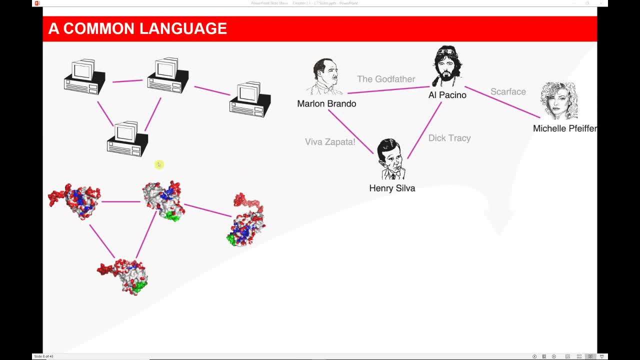 it's appropriate, but in most cases we'll just use the two terms interchangeably. This is the simple language that we'll use in order to describe real networks. You can see here a few different examples. This illustration shows the difference between network and graph- The underlying graph. 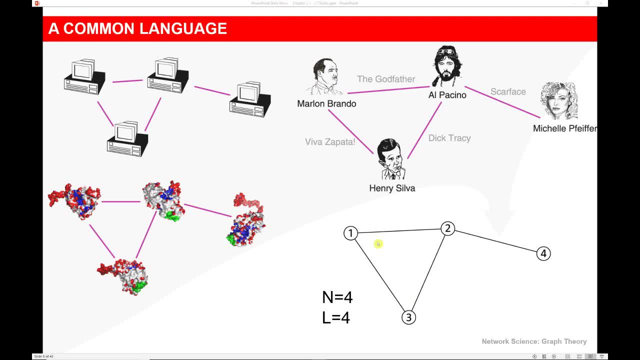 of each of these networks is actually the same. It's a graph of four different nodes and four different edges or links, but we can actually overlay different real-world networks. So if we're looking at a graph of four different nodes, we can see that the node represents a different actor. 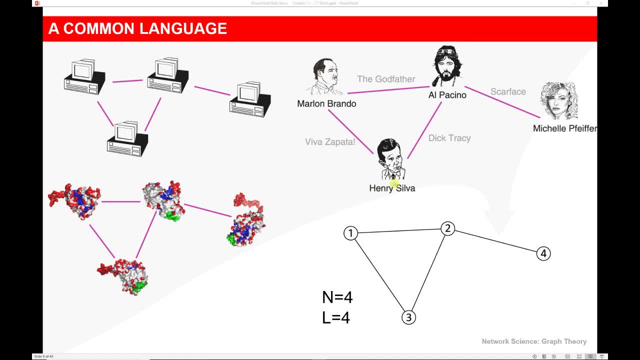 and the link represents a movie in which they both acted. So we can see that each node represents a different actor. So we can see that each node represents a different actor and the link represents a movie in which they both acted. Choosing a network representation is very 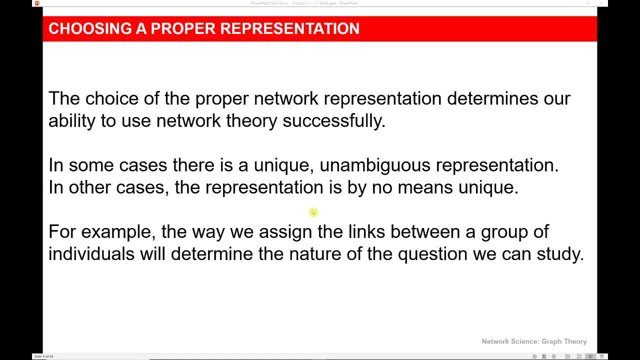 important, as the choice of the proper network representation will determine our ability to use network theory successfully. In some cases there's a unique, unambiguous representation, and I think for most networks in this course, that's what we'll have, But in other cases, 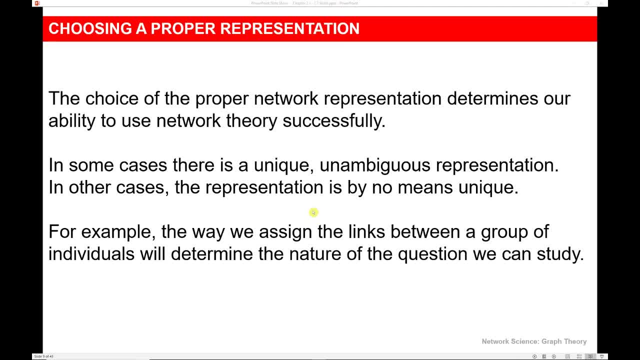 the representation is by no means unique. For example, the way we assign the links between a group of individuals will determine the nature of the question that we can study. For example, I could create a network of all of the faculty in the CIDM department and I would have to decide. 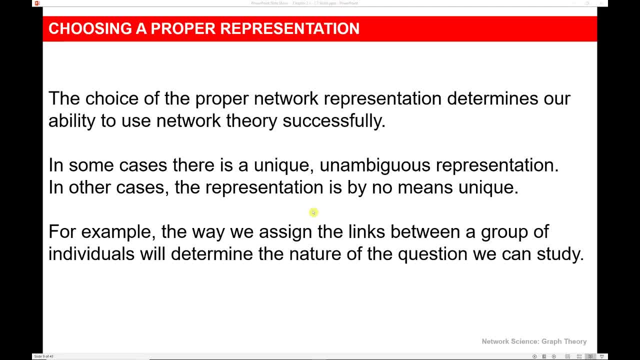 what kind of link I would want between each faculty member. Would the link represent simply that they work together, that they've taught the same course, or perhaps that they've researched together? The choice of the link would determine what kind of analysis we could do with that. 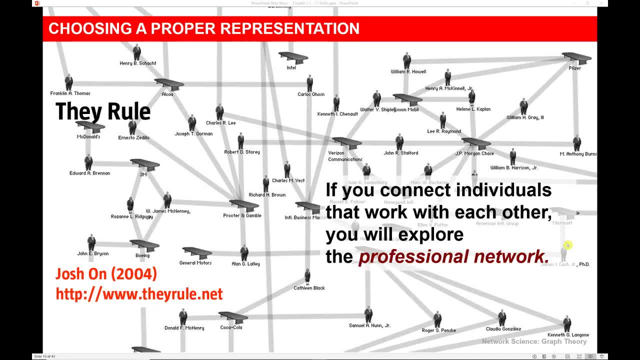 network, A great example of a social network that I encourage you to explore in this course, perhaps for your project. most of you are probably on LinkedIn. You can see that if you connect individuals that work with each other, you're going to explore the professional network. Some network representations might not be as useful. 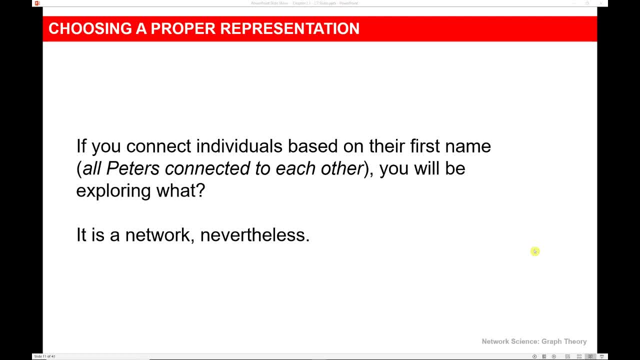 though. For example, if you connect individuals based on their first name, like we connect everybody named Peter, well, we certainly have a network, but I'm not really sure what kinds of things we can explore. It is a network nevertheless. I actually think there are. 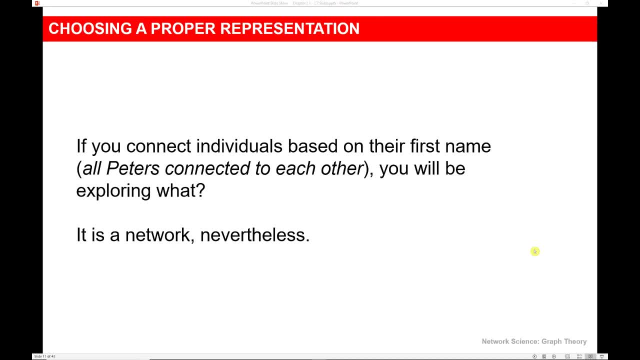 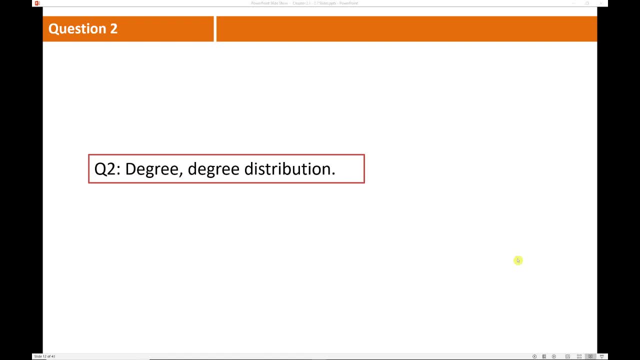 some questions that you could ask about. all the people that are named Peter connected to each other. It would be interesting to see if there's some kind of pattern. When we talk about networks, we'd also like to talk about different properties of nodes. Here we're going to define degree. 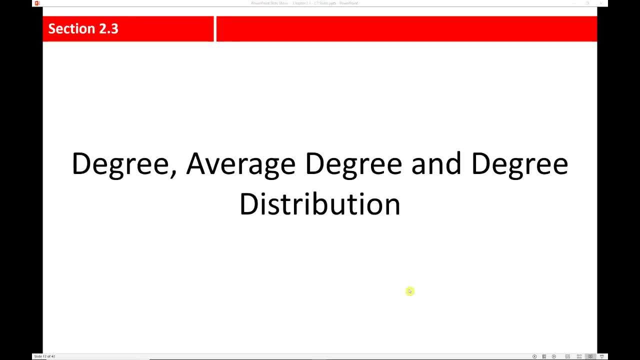 and degree distribution. The degree of a node is going to be the number of edges that are attached to that node, The average degree we can calculate for the entire network. that would answer for us on average how connected is everybody in the network. And if we plot, 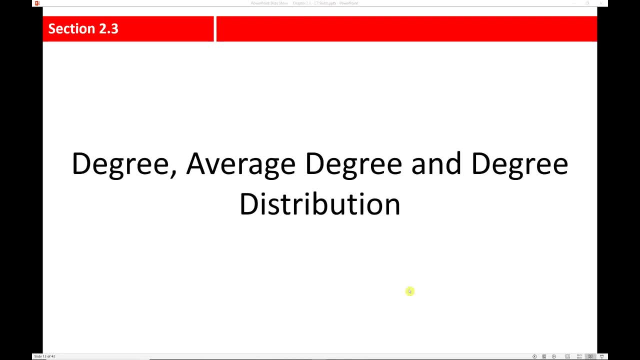 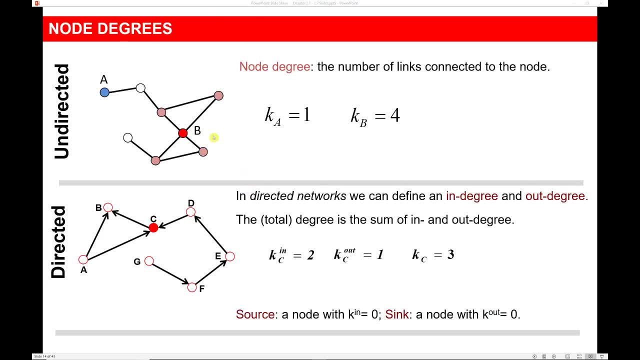 a distribution. we can also look at how many hubs we have in the network, how many people are very connected. Here on the left we have an undirected graph and a directed graph. Let's look at the undirected graph first. You can see it's undirected because we don't have any arrows. So the connection 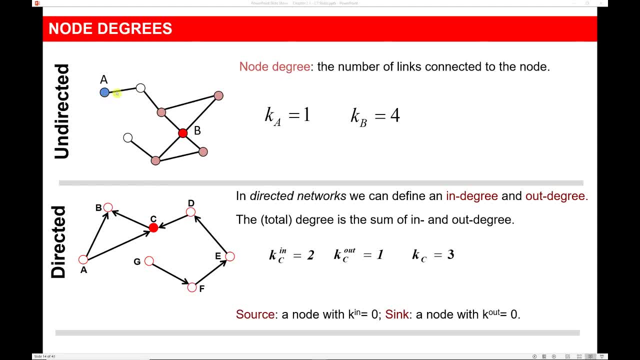 between nodes is the same from one node to the other and vice versa. The degree in an undirected graph is simply the number of links connected to the node. So the degree of node A is one and the degree of node B is four. You can count all of the edges coming out. 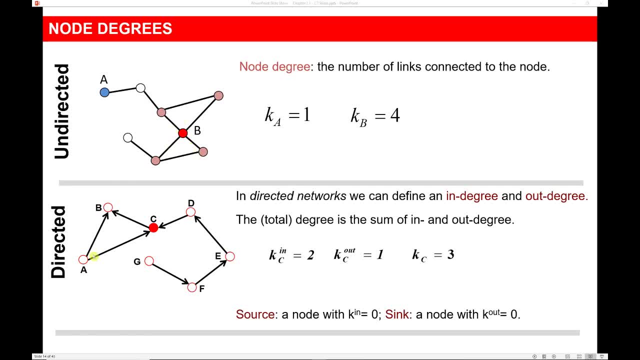 of that node. In a directed network, it's slightly different. First of all, you can see that this network does have direction. So A points to B, but B does not point to A. We would need a directed network to represent Twitter followers, for example, Because maybe person A is following. 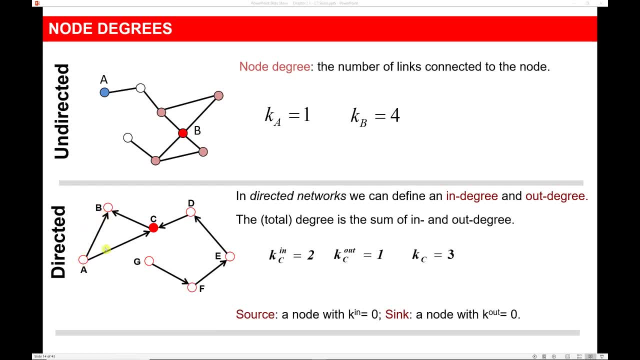 person B, but person B is not following person A. In a directed network we define an in-degree and an out-degree. So an in-degree is how many connections are coming into that node and an out-degree is how many connections are coming out of that node. 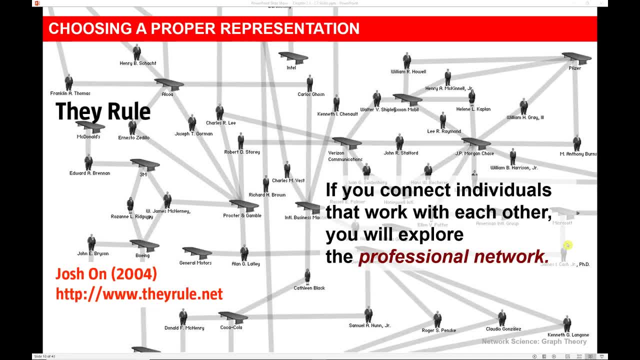 network, A great example of a social network that I encourage you to explore in this course, perhaps for your project. most of you are probably on LinkedIn. You can see that if you connect individuals that work with each other, you're going to explore the professional network. Some network representations might. 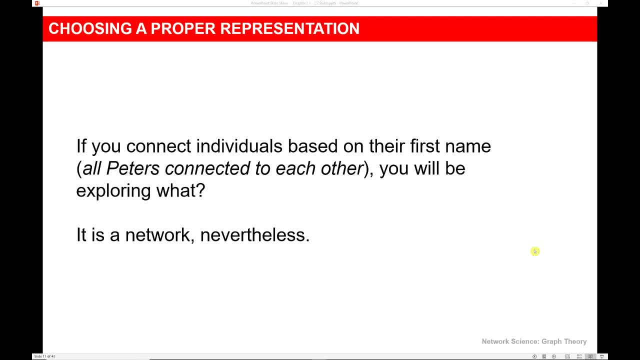 not be as useful though. For example, if you connect individuals based on their first name, like we connect everybody named Peter. well, we certainly have a network, but I'm not really sure what kinds of things we can explore. It is a network nevertheless. I actually 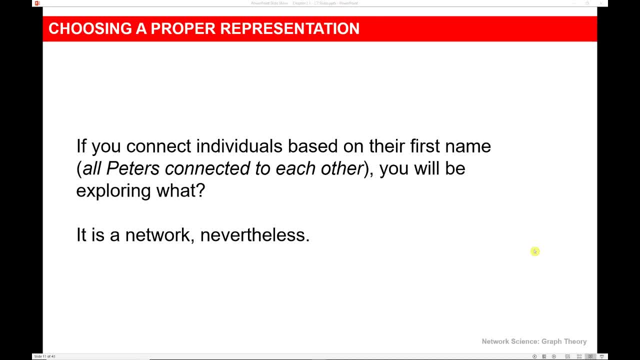 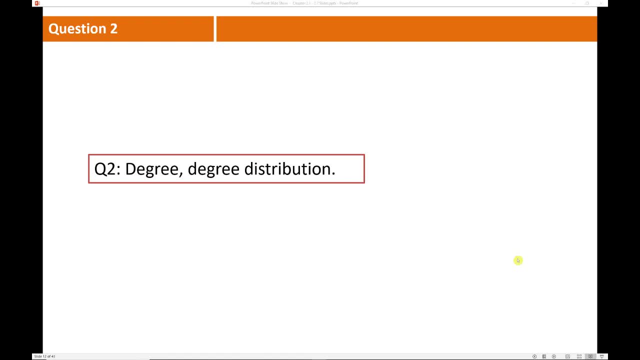 think there are some questions that you could ask about all the people that are named Peter connected to each other. It would be interesting to see if there's some kind of pattern. When we talk about networks, we'd also like to talk about different properties of nodes. Here we're going to define 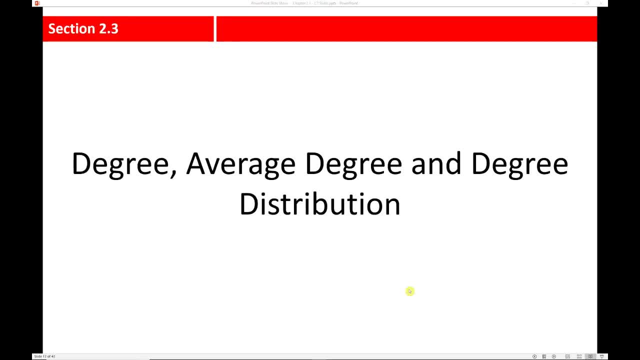 degree and degree distribution. The degree of a node is going to be the number of edges that are attached to that node, The average degree we can calculate for the entire network. that would answer for us on average how connected is everybody in the network. And if we plot, 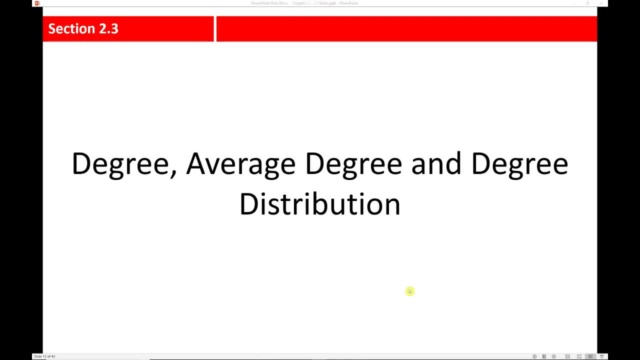 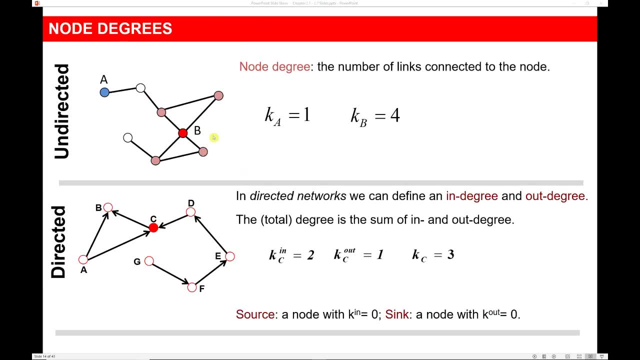 a distribution. we can also look at how many hubs we have in the network, how many people are very connected. Here on the left we have an undirected graph and a directed graph. Let's look at the undirected graph first. You can see it's undirected because we don't have any arrows, The connection between 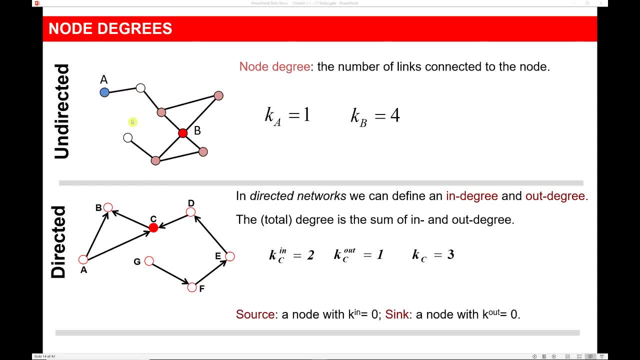 nodes is the same from one node to the other and vice versa. The degree in an undirected graph is simply the number of links connected to the node. The degree of node A is 1, and the degree of node B is 4.. You can count all of the edges coming out of that node In a. 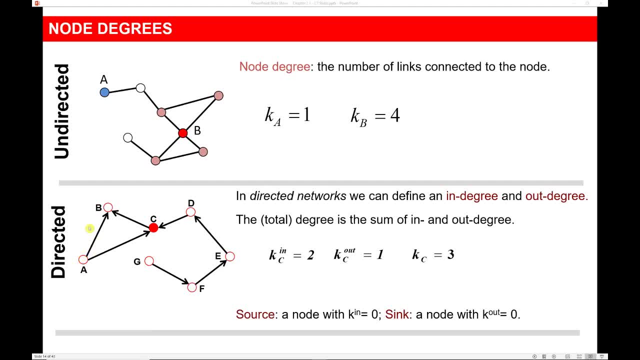 directed network, it's slightly different. First of all, you can see that this network does have direction, so A points to B, but B does not point to A. We would need a directed network to represent Twitter followers, for example, because maybe person A is following. 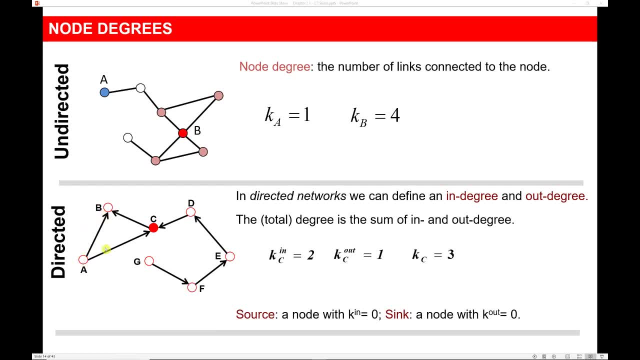 person B, but person B is not following person A. In a directed network we define an in-degree and an out-degree. An in-degree is how many connections are coming into that node, and an out-degree is how many connections are coming out of that node. 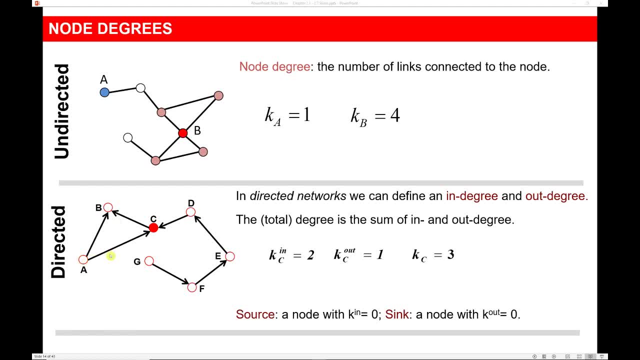 node and to get the total degree you're just going to add both of those together. so if we look at node c, for example, we have two coming in and one going out, so we have an in degree of two and an out degree of one and we have a total degree of three. if we have a node where there's nothing. 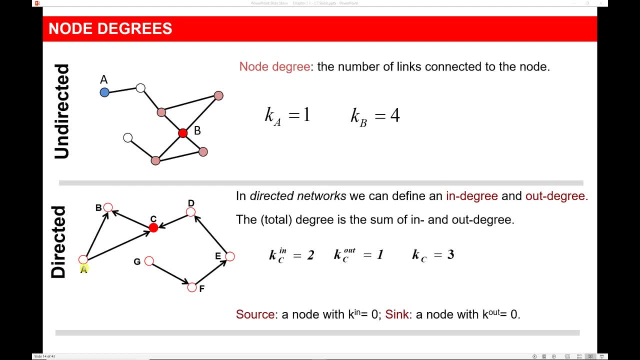 pointing to that node. we have a source node. so for example, node a, we have nothing pointing to it. we have an in degree of zero. that is a source node. and if we have a node like b, where there's nothing coming out of the node, only edges going into the node, then we have a sink. so a sink has out degree. 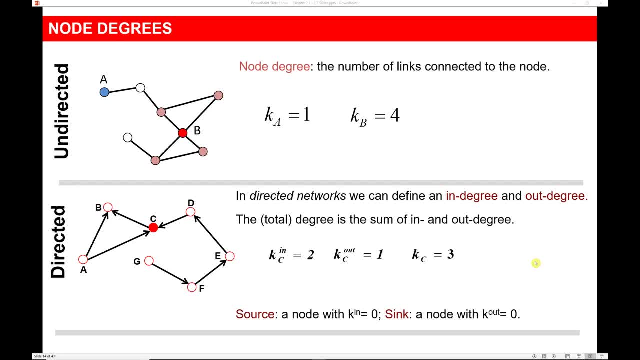 of zero. we can use the degree of nodes as a simple measure of influence within the network. if you think about it, you can probably think of people in your network that are highly connected. those would be the people with the high degree if we have a directed graph like web pages on the internet. 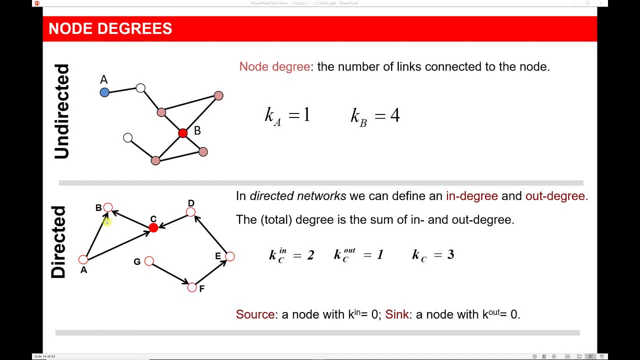 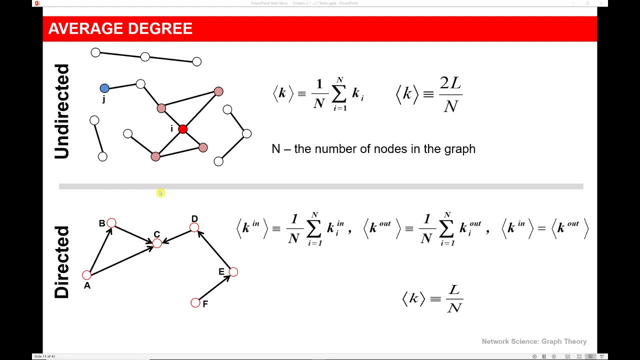 we can consider that a web page that has a lot of links pointing to it, that might be an important node, but we could also have a web page that points to a lot of different pages that could also be important in its own right. in order to calculate the average degree, we just average the total degree. 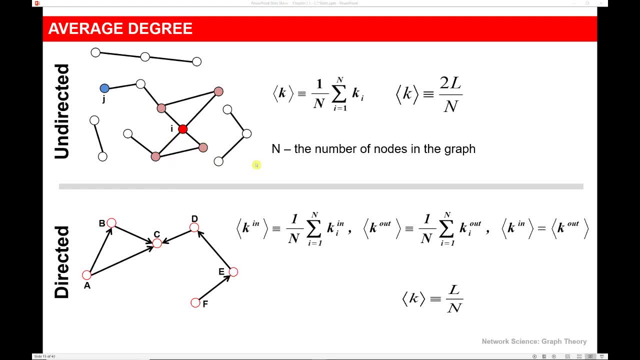 in an undirected graph. we'll show you how to do this in geffy. in a directed graph it's a little bit different because we have both in degree and out degree, but we can calculate the average degree in direction and we can also do a directed graph in geffy as well. here are a few examples of different networks. 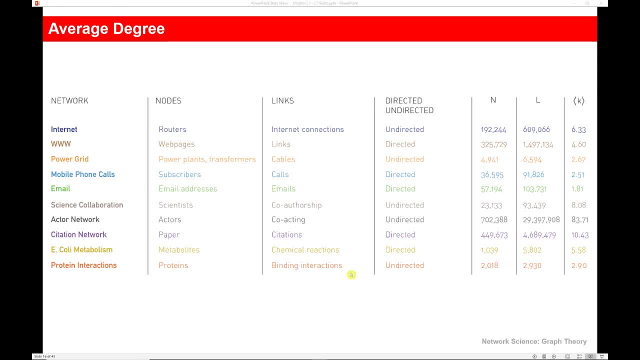 with some simple data about those networks. so, for example, we have the internet where each node is a router and the edges or the links between routers are internet connections. this is an undirected graph, because routers can communicate back and forth at the time this data was obtained. 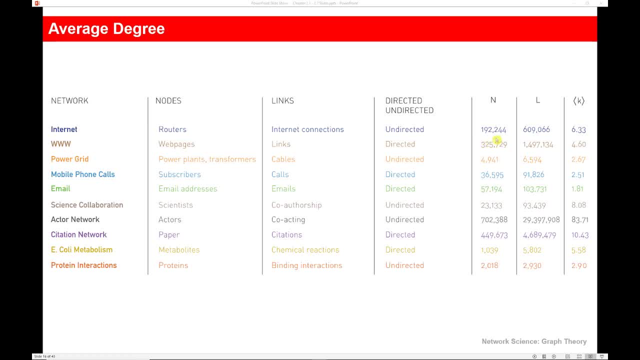 we had about 192 000 nodes or routers in the network and about 609 000 links between them, with, on average, each router being connected to six other routers. if we take a look further down, you can see that in the actor network there were quite a few. 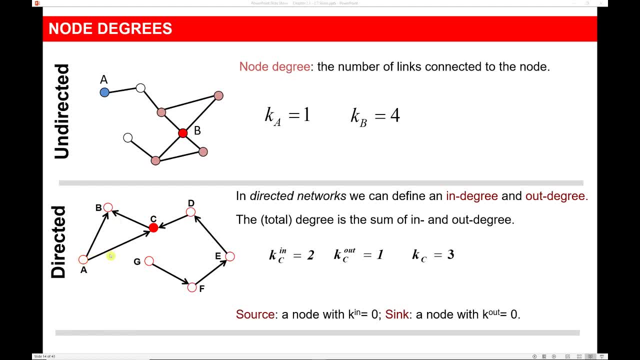 And to get the total degree you're just going to add both of those together. So if we look at node C, for example, we have two coming in and one going out, So we have an in-degree of two and an out-degree of one and we have a total degree of three. 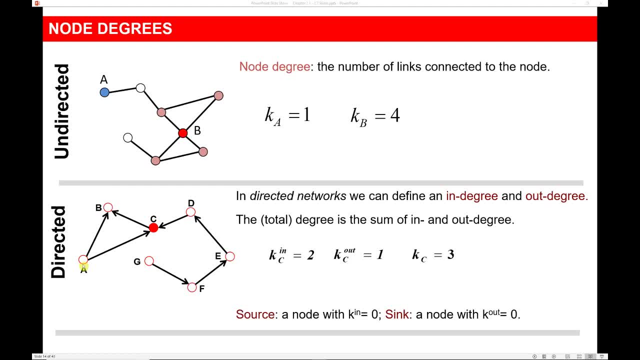 If we have a node where there's nothing pointing to that node, we have a source node. So, for example, node A, we have nothing pointing to it, We have an in-degree of zero. That is a source node. And if we have a node like B, where there's nothing coming out of the node, only edges, 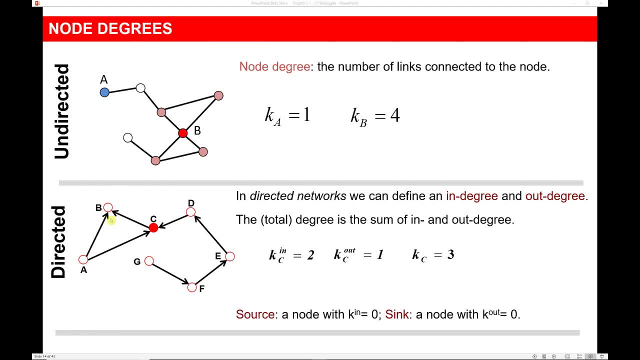 going into the node. then we have aync, so a sync has out-degree of zero. We can use the degree of nodes as a simple measure of influence within the network. If you think about it, you can probably think of people in your network that are highly 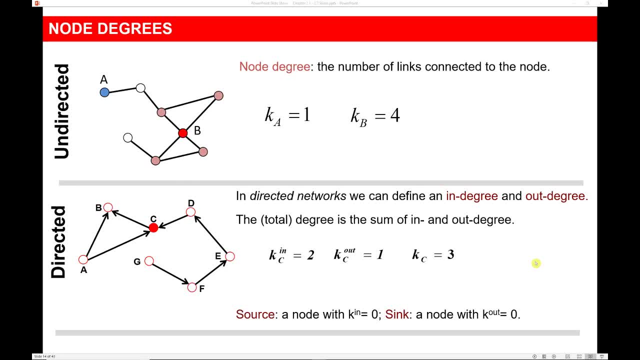 connected. Those would be the people with the high degree. If we have a directed graph like web pages on the Internet, you can consider that a web page has a lot of links around internet So that directly connects to that network, as the network has the most search early link connections. 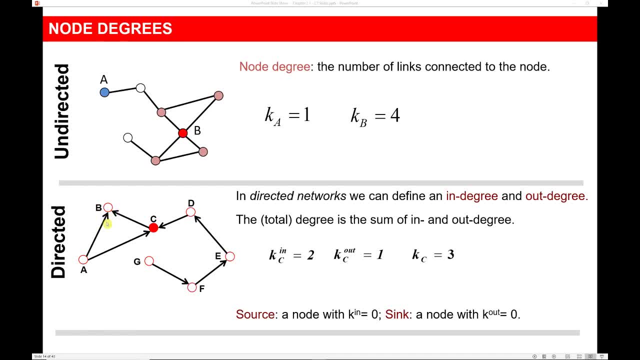 So our definition of a meeting network is turned theoretically. In the case of a web page that, as an example, has different connections due to the 500 links pointing to it, that might be an important node, but we could also have a 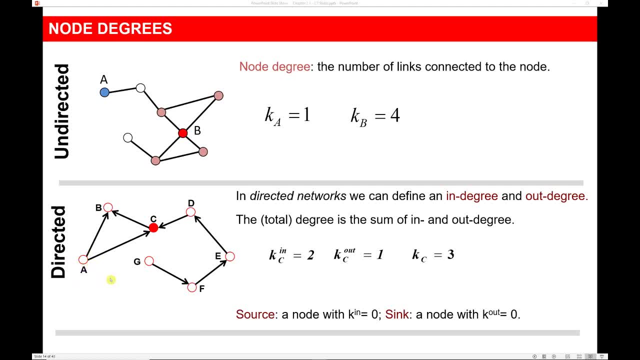 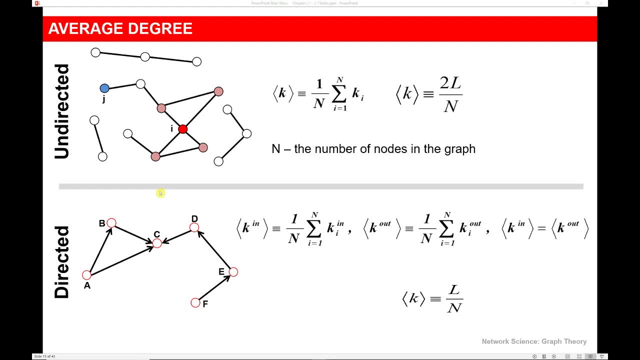 web page that points to a lot of different pages That could also be important in its own right. In order to calculate the average degree, we just average the total degree in an undirected graph. We'll show you how to do this in Gephi. In a directed graph it's a little bit different, because we 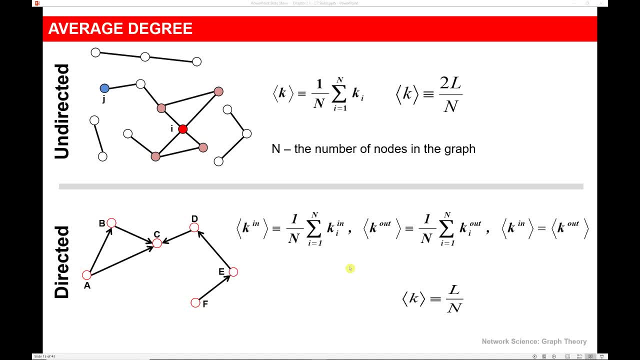 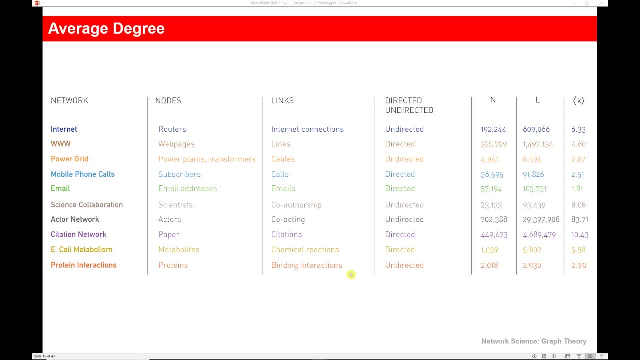 have both in-degree and out-degree, but we can calculate the average degree in directed graph in Gephi as well. Here are a few examples of different networks with some simple data about those networks. For example, we have the internet, where each node is a router and the edges or the links between routers. 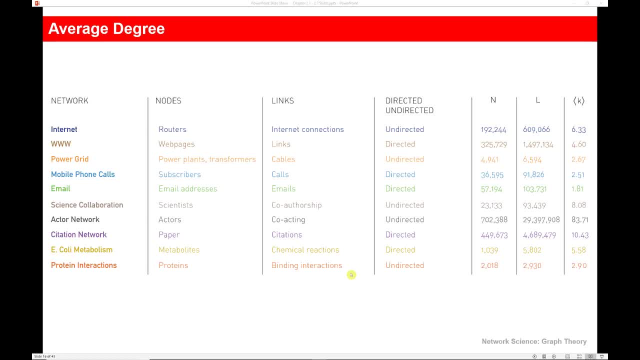 are internet connections. This is an undirected graph, because routers can communicate back and forth. At the time this data was obtained, we had about 192,000 nodes or routers in the network and the data was obtained in Gephi. We have about 609,000 links between them with, on average, each router being 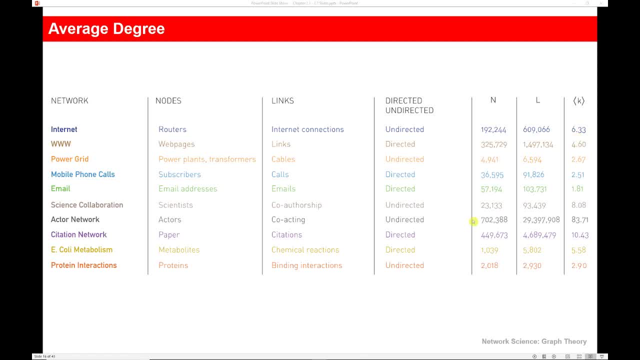 connected to six other routers. If we take a look further down, you can see that in the actor network there were quite a few based on who is in the Screen Actors Guild and quite a few links between different actors that worked in the same movie. This data here tells us that each actor is connected to 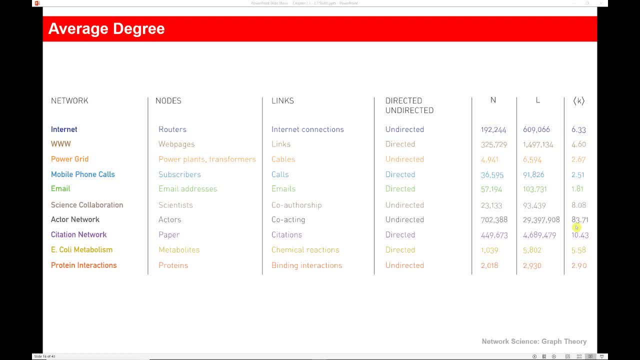 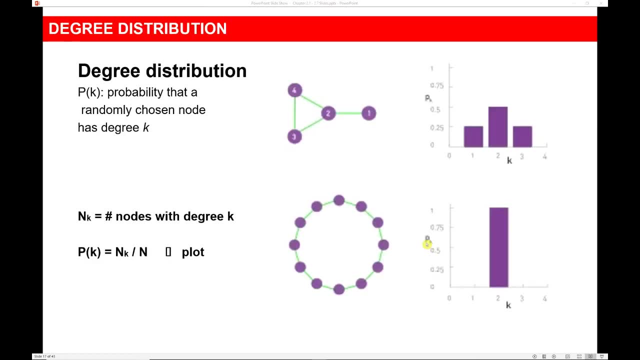 83 other actors. This kind of makes sense, because most movies have a lot of different actors And perhaps they also have a lot of the same actors. We can also talk about the distribution of degree in a network. So in other words, if I choose a node, 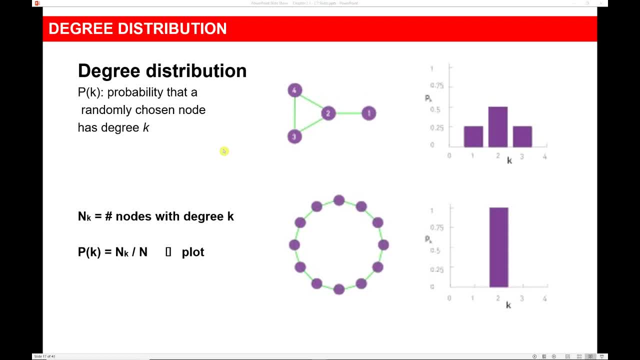 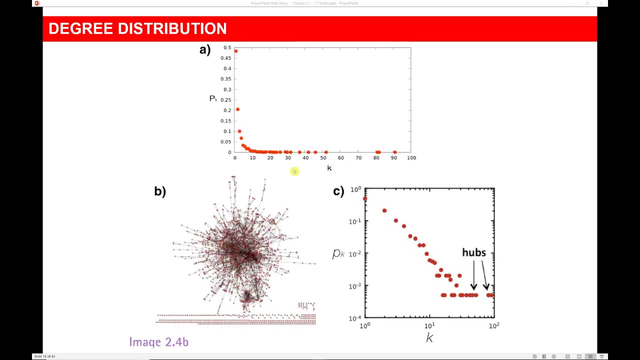 randomly from the network. what's the probability that it will have a particular degree? And, as Barbashi mentioned, we mostly have nodes that only have a few different connections because most people are connected and will have very few hubs. If we take a look, this graph here shows that representation very well. 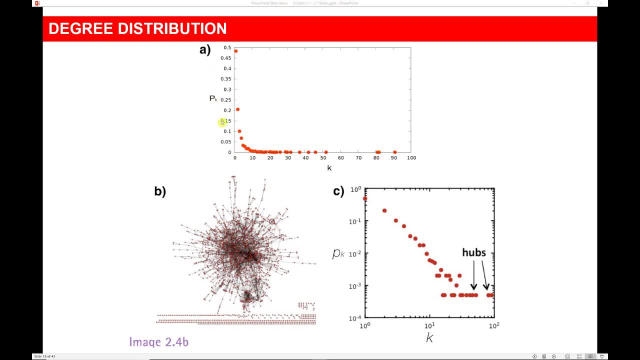 So on the y-axis, we have the probability that if we pick a node, it will have a particular degree. This would be that degree. What this tells us is that the probability of picking a node in this network with a number of connections of 90 is pretty slim, but the probability of finding a node with only a few. 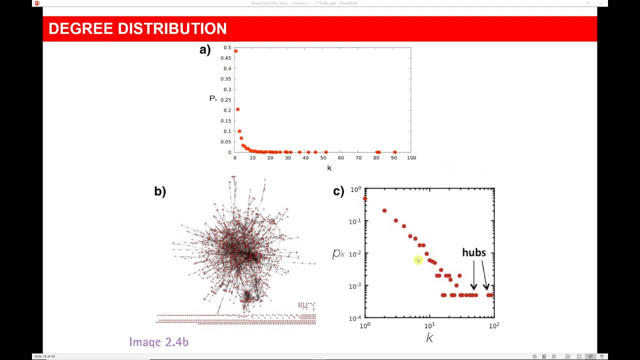 connections is pretty high. This is another statistical way of modeling this and this is the network of interest. So again, the takeaway from here is that typically we're going to find just a few hubs and mostly everybody is going to only have a couple of links in a network that we have. 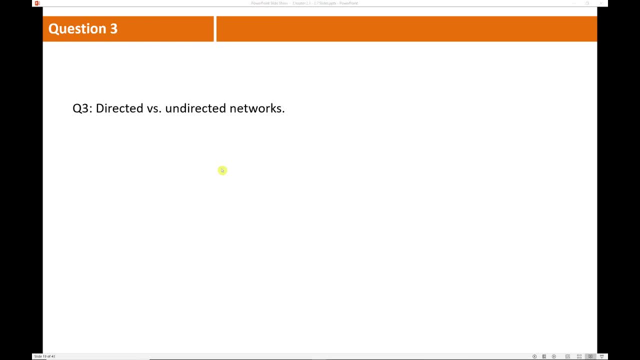 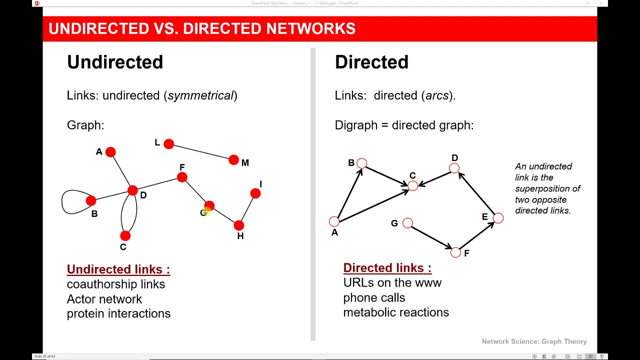 We briefly mentioned directed and undirected networks. let's take a closer look. In an undirected graph the connections are symmetrical. So if I have a connection, for example, from node F to node G, it's the same connection from node G to node F. If we see behavior like this with 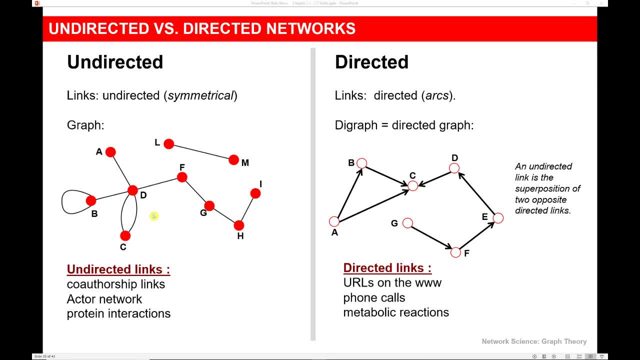 multiple edges from one node to the other in an undirected graph, it's likely that this edge represents a different type of relationship than this edge. We can also have a case where a node is connected to itself, For example, if you had some kind of evaluations. 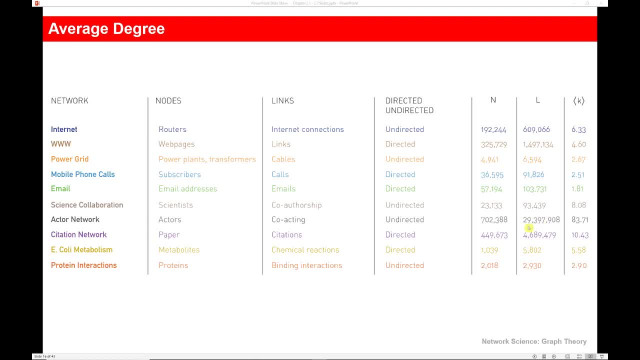 based on who was in the screen actors guild and quite a few links between different actors that worked in the same movie. this data here tells us that each actor is connected to 83 other actors. this kind of makes sense, because most movies have a lot of different actors and perhaps they also have a lot of the same actors we can also talk about. 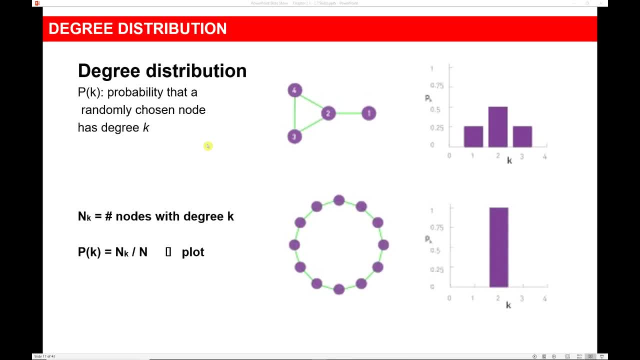 the distribution of degree in a network. so, in other words, if i choose a node randomly from the network, what's the probability that it will have a particular degree? and, as barbashi mentioned, we mostly have nodes that only have a few different connections, because most people are connected and will have very few hubs. if we take a look, this graph here shows that. 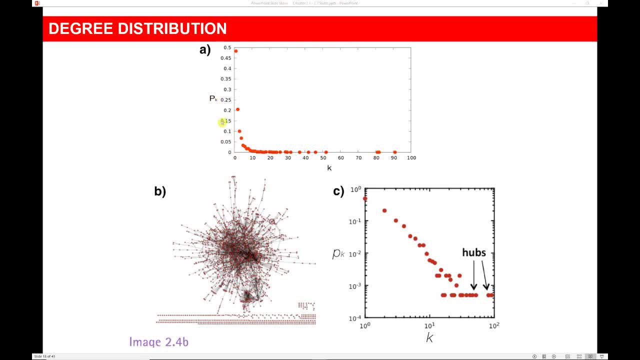 completely不知道 if exactly the node has one node, which office is, because we know that just because there's one node can be one node, or just because a node is a deposit. So again, the takeaway from here is that typically we're going to find just a few hubs and mostly 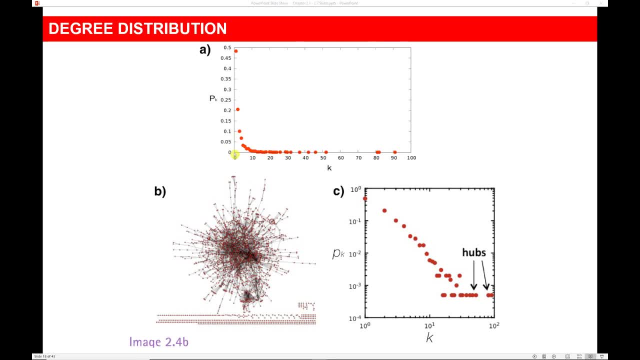 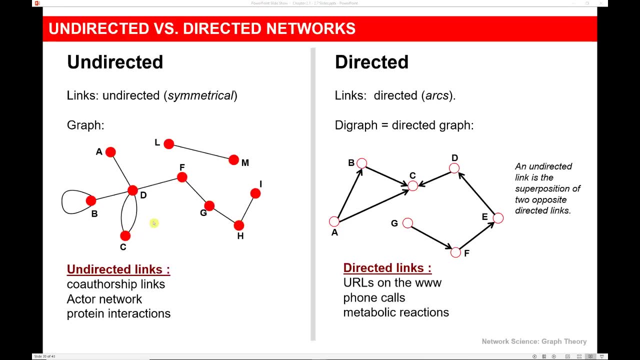 everybody's going to only have a couple of links in a network that we have. We briefly mentioned directed and undirected networks. Let's take a closer look. In an undirected graph the connections are symmetrical. So if I have a connection, for example, from node F to node G, it's the same connection. 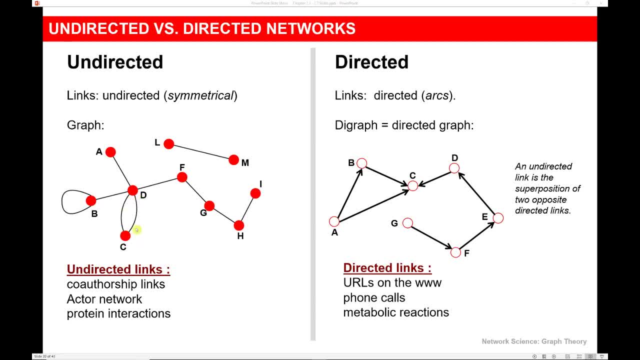 from node G to node F. If we see behavior like this, with multiple edges from one node to the other in an undirected graph, it's likely that this edge represents a different type of relationship than this edge. We can also have a case where a node is connected to itself. 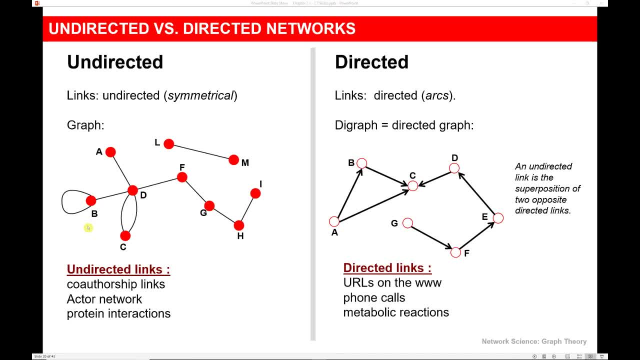 For example, if you had some kind of evaluations in your company and somebody got to evaluate themselves, that might represent that Undirected graphs can be used for representing co-authorship or actors that have acted in the same movies Or protein interactions In a directed graph. we might have some asymmetry. 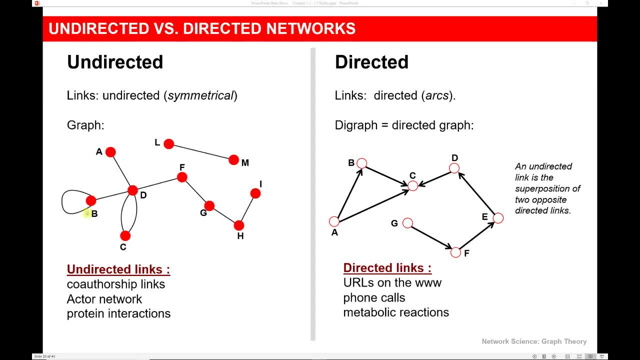 in your company and somebody got to evaluate themselves. that might represent that Undirected graphs can be used for representing co-authorship or actors that have acted in the same movies or protein interactions. In a directed graph we might have some asymmetry. So in other words, 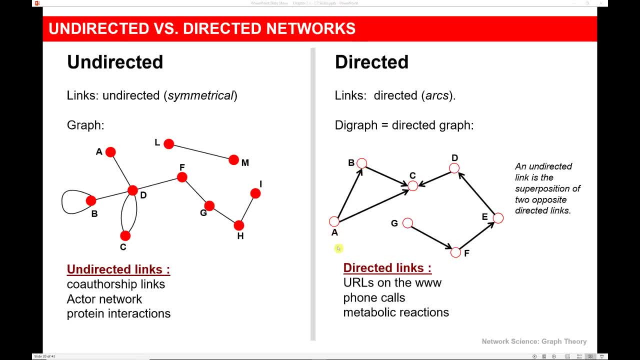 just because A points to B, B might not point to A. In a directed graph, we usually refer to the edges as arcs instead of edges, And the shorthand is referring to the graph as a digraph or directed graph. And, if you think about it, an undirected link is just two opposite directed links. So 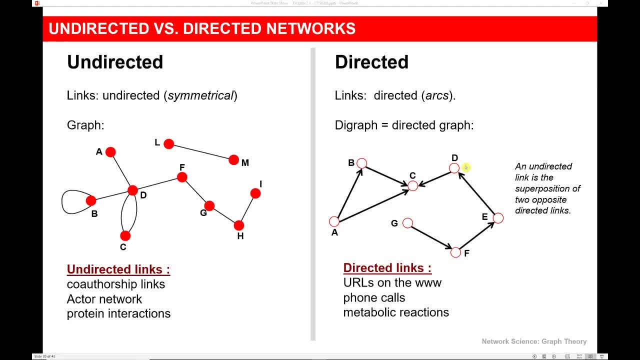 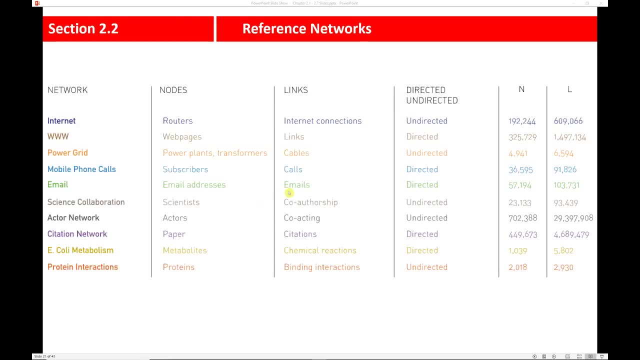 if we have from E to D in an undirected graph, we would also have from D to E. Directed graphs are pretty common, like web pages on the internet or phone calls. Here we can point out some of the different reference networks that are available that are directed. For example, if we have a network of 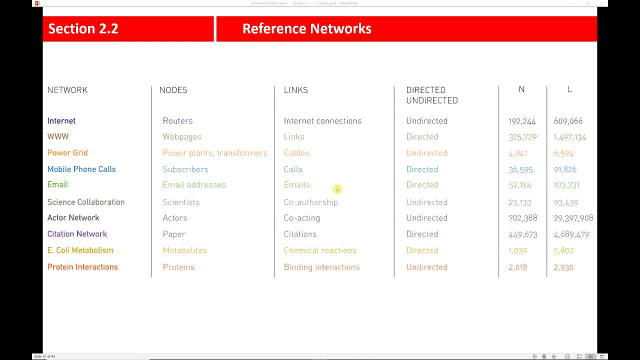 emails- some people may have emailed others and others not emailed them back- Or a mobile phone call network where some people called other people but maybe they didn't get calls back. You can take a look at how the different number of links varies in these directed networks as compared to the number of nodes. 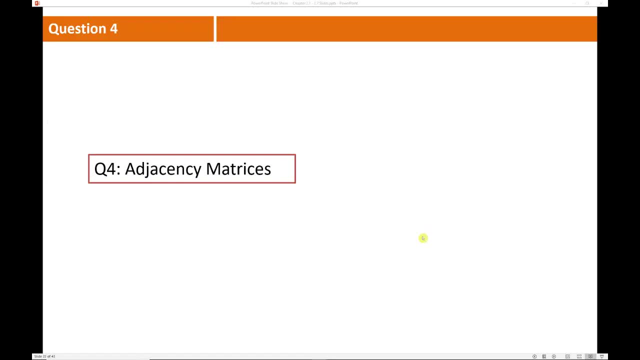 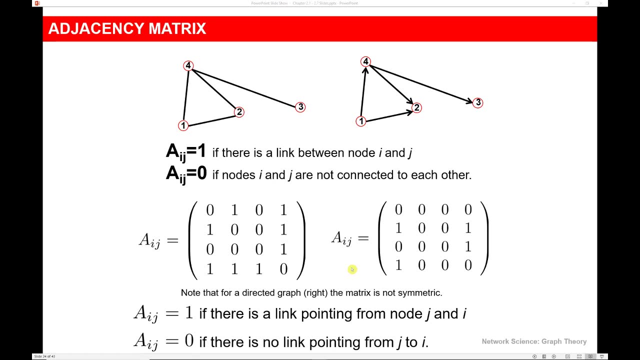 The most common way to represent data in a graph is what's called an adjacency matrix. It's likely that you'll come across an adjacency matrix in this course when you're working with data. What is an adjacency matrix and what does it look like? 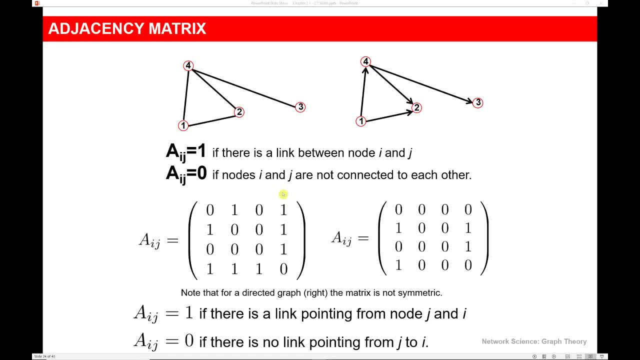 Here we have two examples of adjacency matrices: On the left we have an undirected example and on the right we have a direct example. The adjacency matrix will have a one wherever there's a connection between two nodes. Since we have four nodes in the graph, we have both four rows and 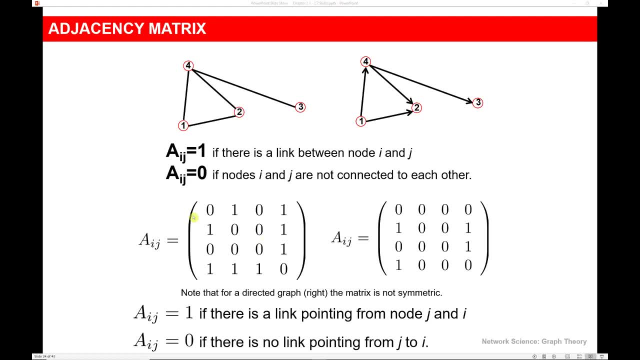 four columns in the adjacency matrix. If you think about it, that means that we have the possibility of 16 different links. If we had ones in every single one of these spaces, that would mean that we have a complete graph, or a graph where every node is connected to every other node. The way we 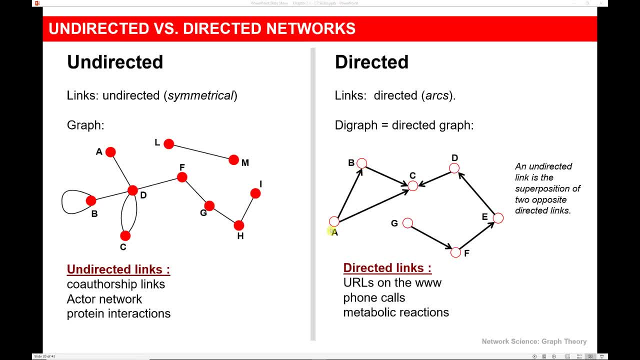 So, in other words, just because A points to B, B might not point to A. In a directed graph, we usually refer to the edges as arcs instead of edges, And the shorthand is referring to the graph as a digraph or a directed graph. 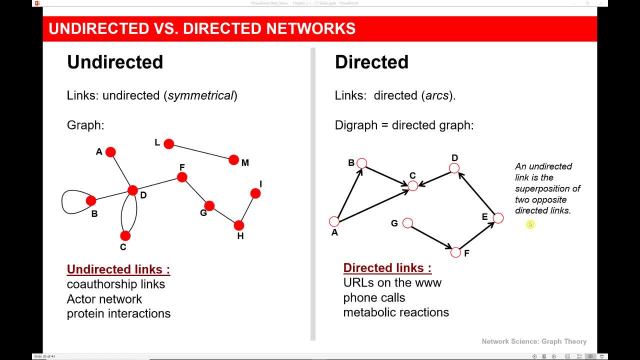 And, if you think about it, an undirected link is just two opposite directed links. So if we have from E to D in an undirected graph, we would also have a directed link, And if we have from D to E, directed graphs are pretty common, like webpages on the internet. 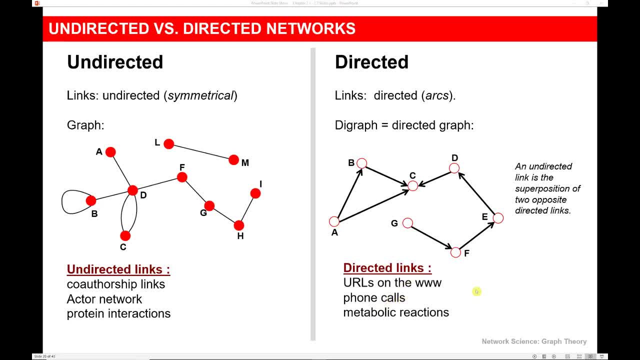 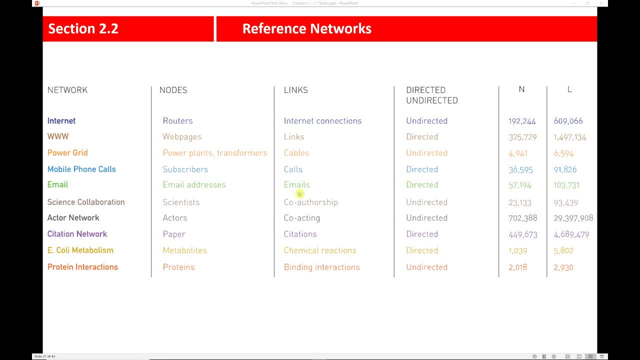 or phone calls that have been placed, Twitter or metabolic reactions. Here we can point out some of the different reference networks that are available that are directed. For example, if we have a network of emails, some people may have emailed others and others. 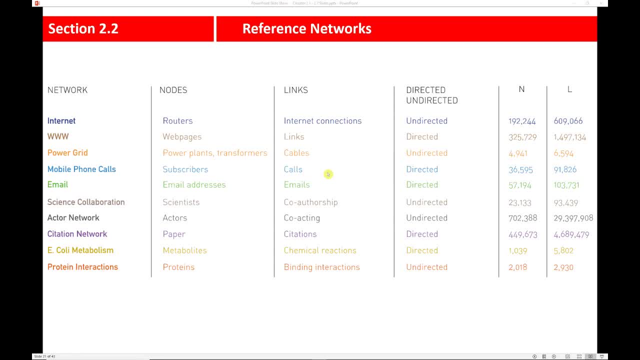 not emailed them back. Or a mobile phone call network where some people called other people but maybe they didn't get calls back. You can take a look at how The different number of links varies in these directed networks as compared to the number of nodes. 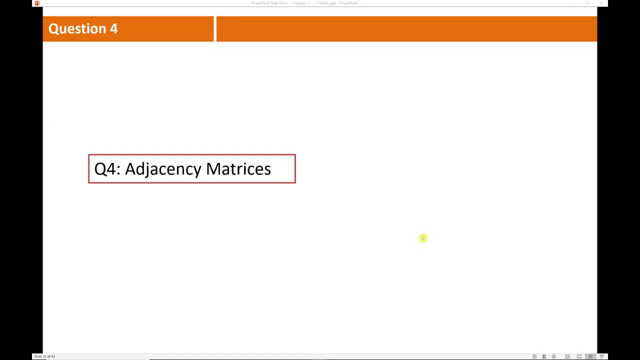 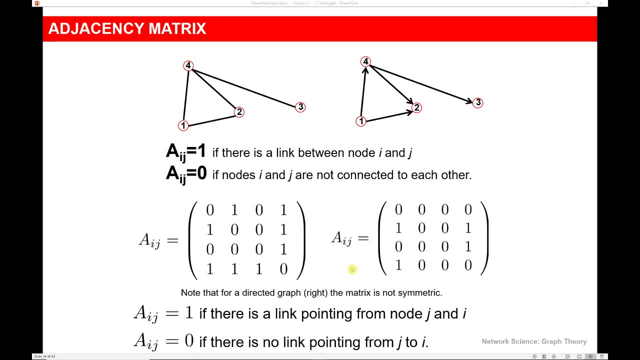 The most common way to represent data in a graph is what's called an adjacency matrix. It's likely that you'll come across an adjacency matrix in this course when you're working with data. What is an adjacency matrix and what does it look like? 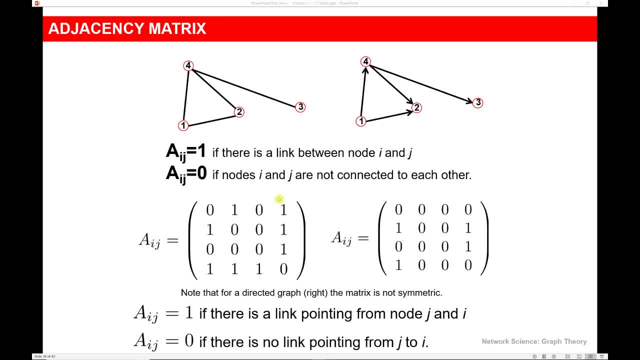 Here we have two examples of adjacency matrices: On the left we have an undirected example, And on the right we have a direct example. The adjacency matrix will have a one wherever there's a connection. Since we have four nodes in the graph, we have both four rows and four columns in the 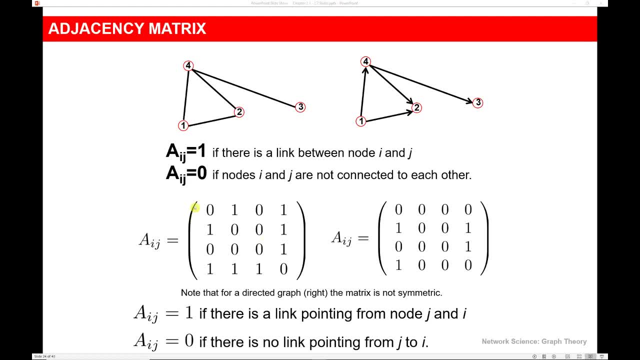 adjacency matrix. If you think about it, that means that we have the possibility of 16 different links. If we had ones in every single one of these spaces, that would mean that we have a complete graph, or a graph where every node is connected to every other node. 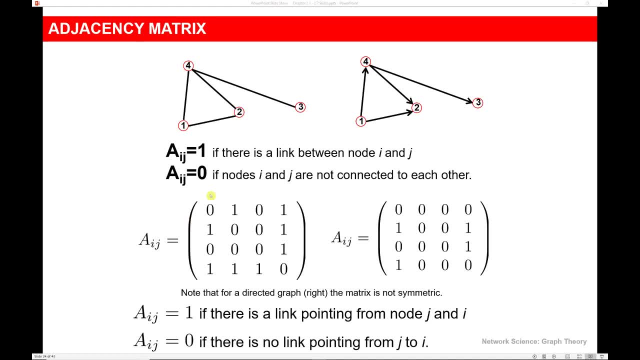 The way we read this is column first and then row. So this column indicates which nodes node one is connected to. This column indicates which nodes node two is connected to Node three and node four. We read this saying that we have edge one, two in this graph. 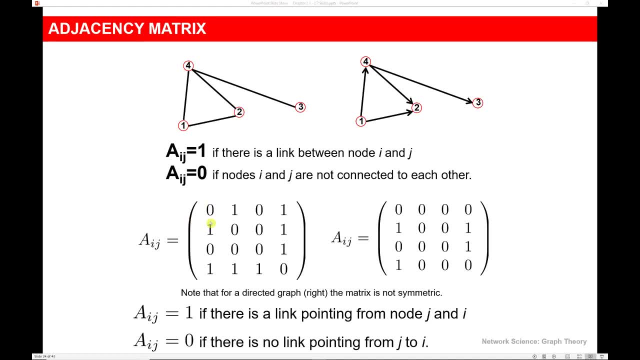 read: this is column first and then row, So this column indicates which nodes node one is connected to. This column indicates which nodes node two is connected to Node three and node four. We read this saying that we have edge one, two in this graph, So node one is connected to node two. 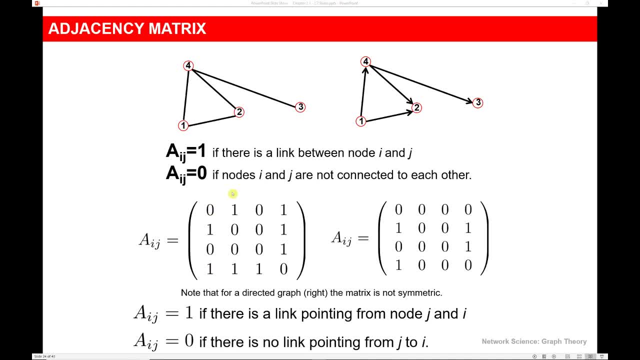 Node one is also connected to node four. If we start in this column we have the different connections for node two. So we have node two is connected to node one as well as node two is connected to node four. Notice that in the undirected case we have 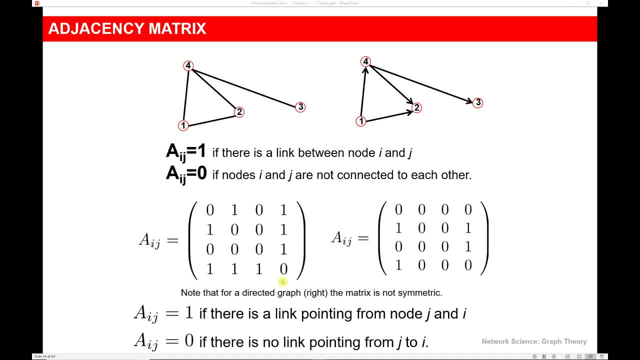 symmetry across this diagonal line, because if there's a connection one way, there's a connection, assumed to be, the other way around as well. If we look at the directed adjacency matrix, we don't have this symmetry. We would only have the symmetry if we had arrows pointing both ways for each edge. but we interpret this in 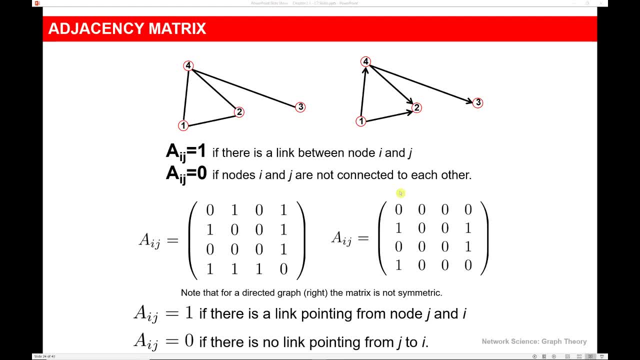 the exact same way. So here we can see that we have a connection from node 1 to node 2 and from node 1 to node 4.. We also have a connection from node 4 to node 2 and from node 4 to node 3.. And 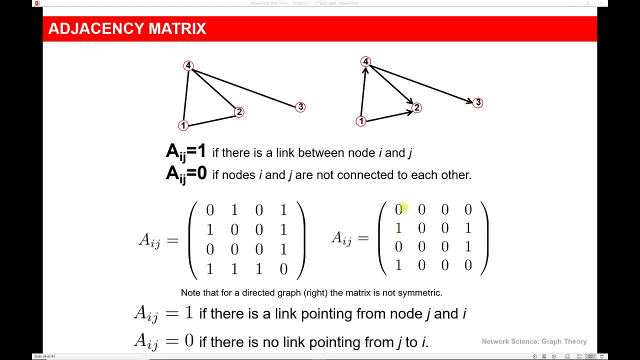 again, this is not symmetric, because even though we have 1 to 2, we do not have 2 to 1.. So, again, there's a 0 every place that there's no edge and there's a 1 every place that there is an edge. 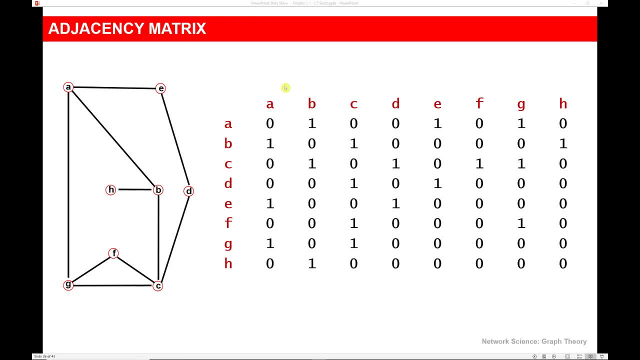 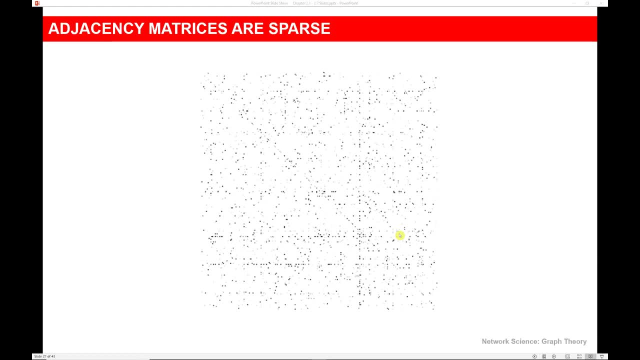 Here is a larger example of an adjacency matrix. The adjacency matrix gets larger the more nodes that you have in the network. Most adjacency matrices are sparse, meaning that there aren't a lot of 1s, because there aren't really that many connections in the graph. If you think about some. 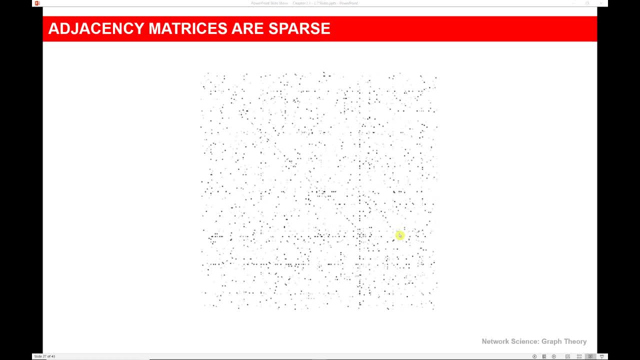 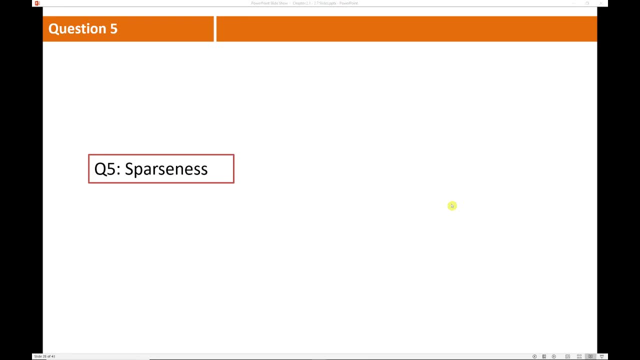 examples of real-world networks. you'll see that this is true. Typically, you don't have complete graphs or cases where everybody is connected to every other person in the network. So we have this characteristic of sparseness, And real networks are sparse. On the right we have an example of what's called a complete graph. 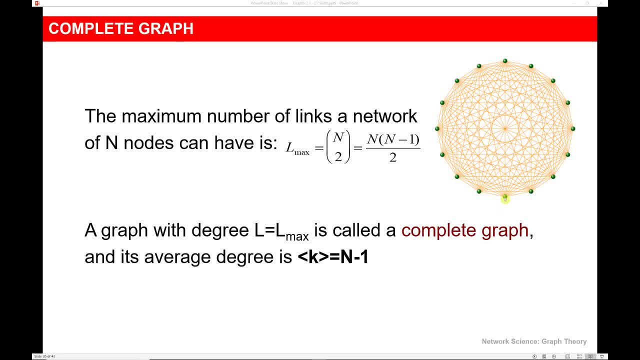 In a complete graph. if you choose a node, that node is going to be connected to every other node in the graph, And if you wanted to calculate the total number of edges in a complete graph, you could use this formula. If the maximum number of possible links is used in a graph, 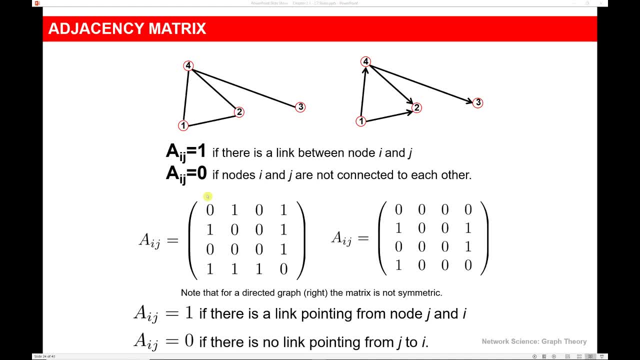 So node one is connected to node two. Node one is also connected to node four. If we start in this column, we have the different connections for node two. So we have node two is connected to node one as well as node two is connected to node four. 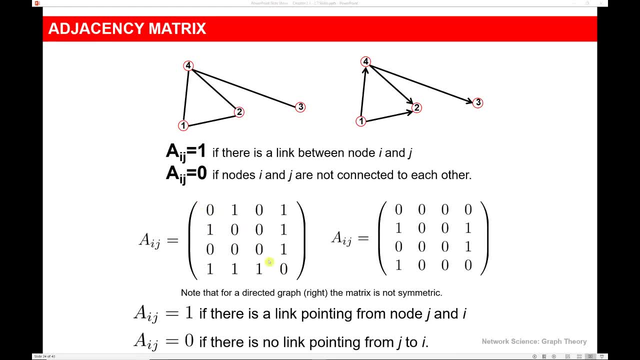 Notice that in the undirected case we have symmetry. We have symmetry across this diagonal line because if there's a connection one way, there's a connection assumed to be the other way as well. If we look at the directed adjacency matrix, we don't have the symmetry. 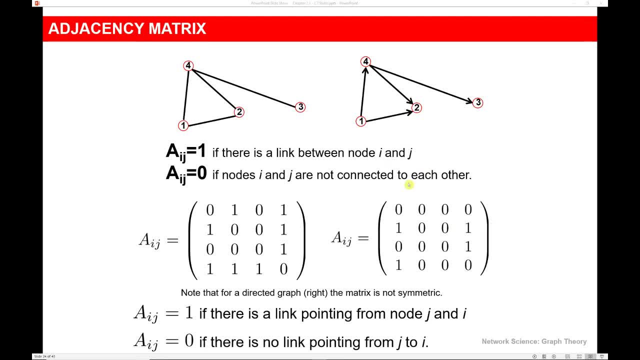 We would only have the symmetry if we had arrows pointing both ways for each edge, but we interpret this in the exact same way. So here we can see that we have a connection from node one to node two and from node one to node four. 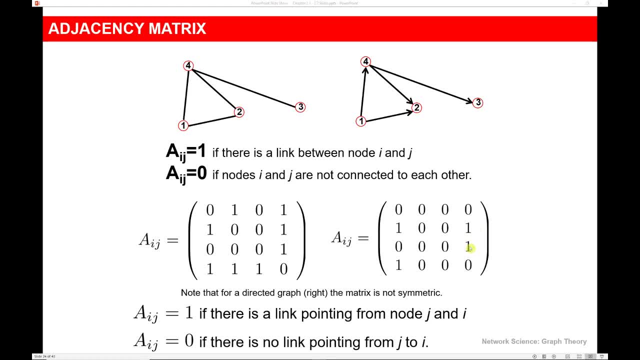 We also have a connection from node four to node two and from node four to node three. And again this is not the same, It's not symmetric, because even though we have one to two, we do not have two to one. So again, there's a zero every place that there's no edge, and there's a one every place. 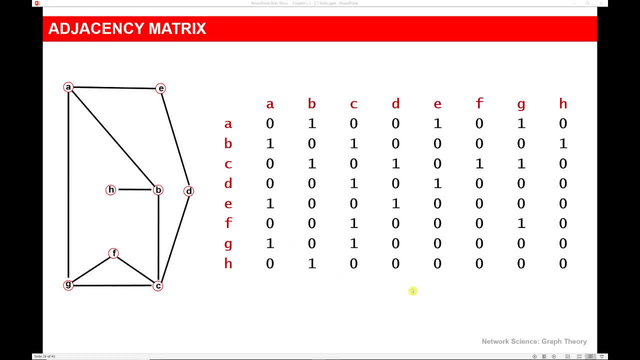 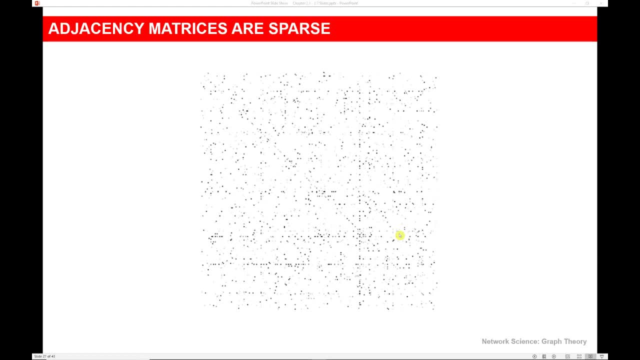 that there is an edge. Here is a larger example of an adjacency matrix. The adjacency matrix gets larger the more nodes that you have in the network. Most adjacency matrices are sparse, meaning that there aren't a lot of ones because there aren't really that many connections in the graph. 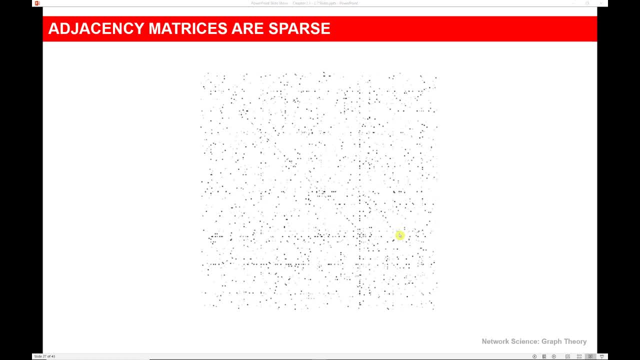 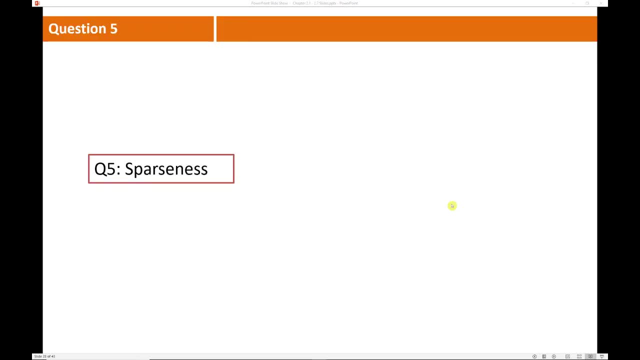 If you think about some examples of real world networks, you'll see that this is true. Typically, you don't have complete graphs Or cases where everybody is connected to every other person in the network, So we have this characteristic of sparseness. 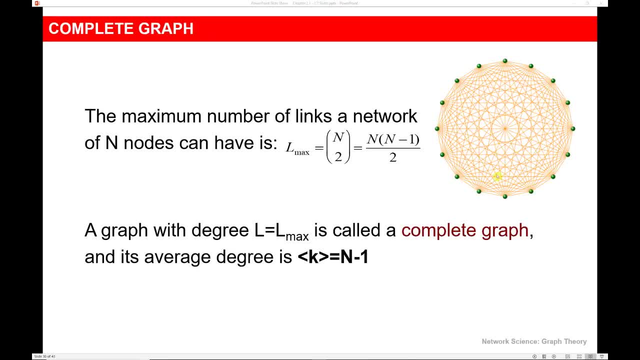 And real networks are sparse. On the right we have an example of what's called a complete graph. In a complete graph, if you choose a node, that node is going to be connected to every other node in the graph. And if you wanted to calculate the total number of edges in a complete graph, you could use this. 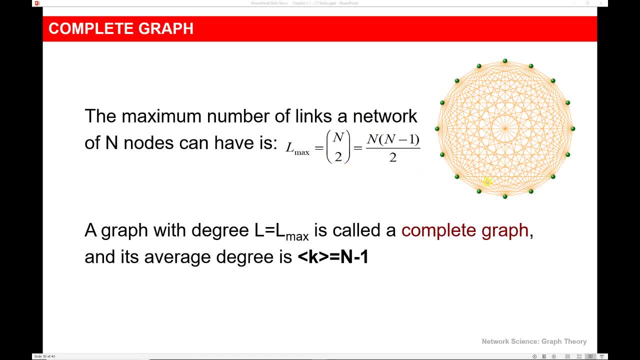 formula. If the maximum number of possible links is used in a graph, it's a complete graph And its average degree can be calculated as zero. So that's one minus the total number of nodes in the graph. If you have a complete network, you can easily calculate the average degree in that network. 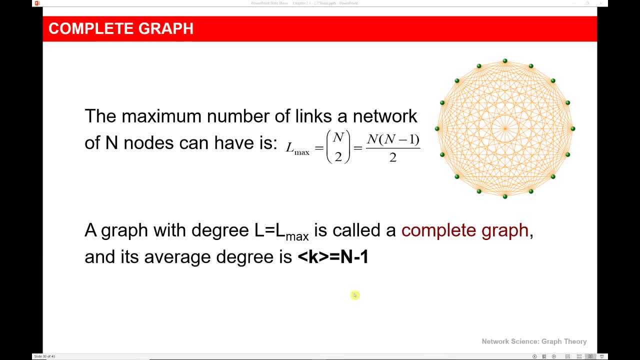 it's a complete graph And its average degree can be calculated as 1 minus the total number of nodes in the graph. If you have a complete network, you can easily calculate the average degree in that network. If we take a look at these real-world examples and their data, 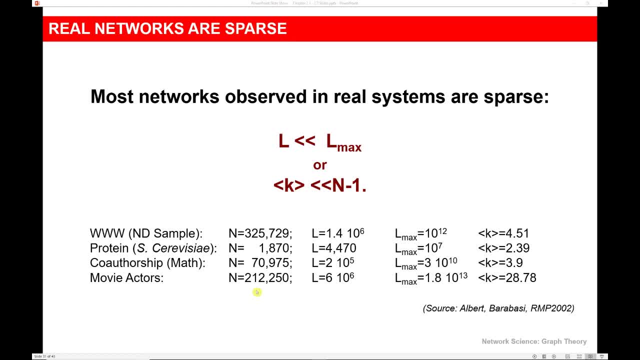 we can see that real networks are sparse. For example, take a look at this movie actor network. We have around 200,000 nodes, so about 200,000 actors, And we only have 6 times 10 to the power of 6 links in the network, which, considering how many nodes there are, isn't that many, Because here 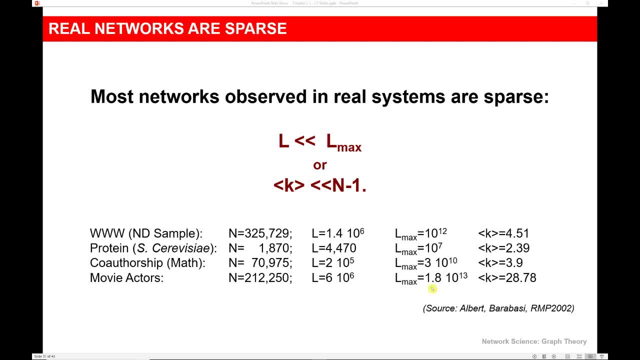 we can see that the maximum number of possible links, which would mean that every actor in the network had acted in at least one movie with a total of 200,000 actors, is a total of 200,000. Every other actor would be 1.8 times 10 to the power of 13.. So you can see that the number of 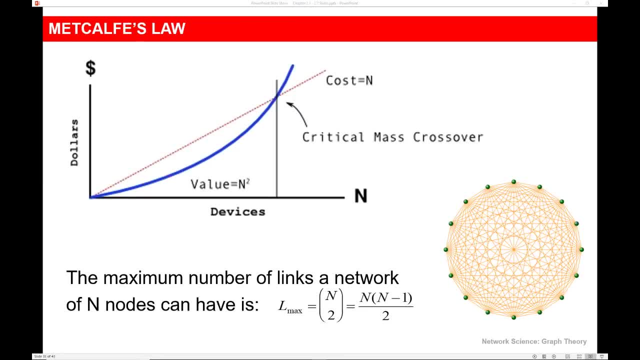 links is way less than the maximum possible number of links. If you haven't heard of Metcalfe's law, Metcalfe's law states that the value of a network is proportional to the square of the number of its nodes. Metcalfe formulated this around 1980, based on the different networks that communication. 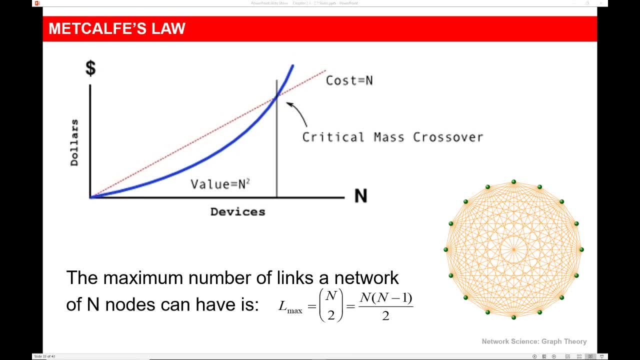 devices were starting to generate at that time And in the late 1990s this was used as a valuation for internet companies. So he suggested that the value of a network is based on the square of the number of nodes, but the cost of using that network was just the number of nodes And 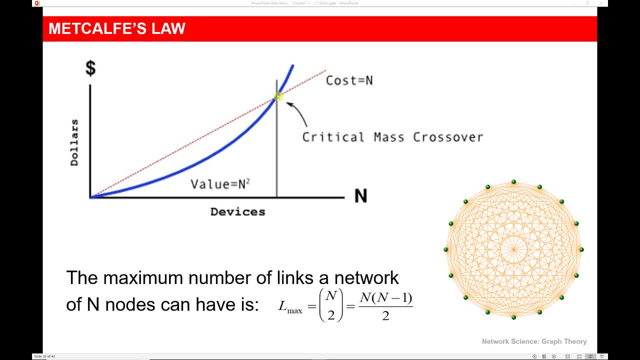 the point at which these two values met- the cost and the value of the network. that was where critical mass was reached and the network would start to become profitable. You can think about Mark Zuckerberg making Facebook and after he started adding advertising to each page. 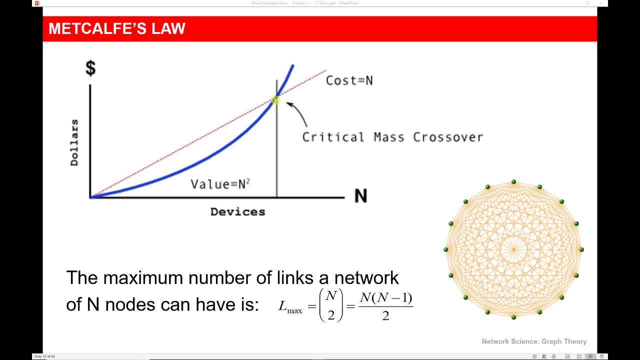 he would generate more revenue the more people were involved with the social network. The truth is, though, because we know that networks, for the most part, are sparse, the value of the network's not actually going to follow this curve. It's going to follow the cost curve. So this is a case. 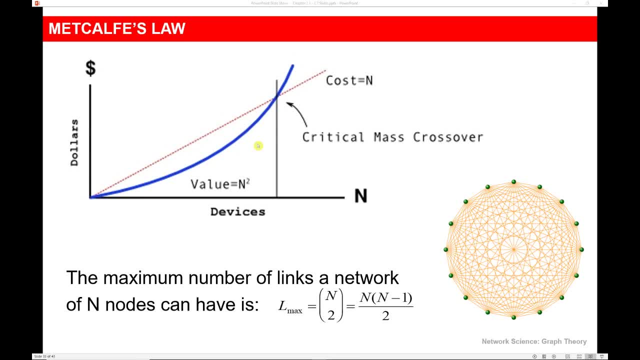 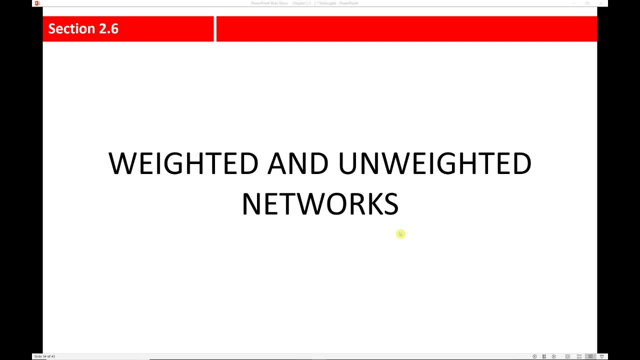 where the real world behavior of networks can inform us as to when a network actually becomes valuable. Network edges can also have weights, So we can have both weighted and unweighted networks. So far we've been looking at networks that are unweighted. 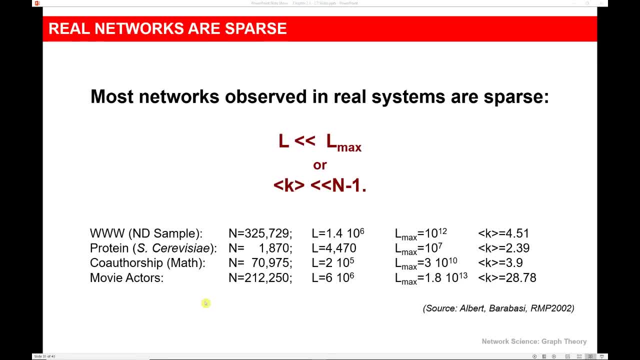 If we take a look at these real world examples and their data, we can see that real networks are sparse. For example, take a look at this movie actor network. We have around 200,000 nodes, So about 200,000 actors. 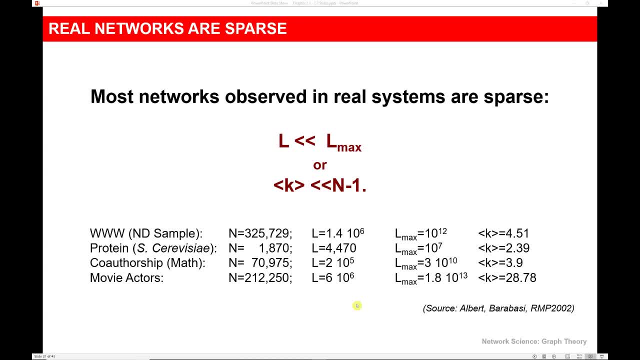 And we only have six times 10 to the power of six links in the network which, considering how many nodes there are, isn't that many, Because here we can see that the maximum number of nodes in the graph is zero. So we can see that the maximum number of possible links, which would mean that every actor in 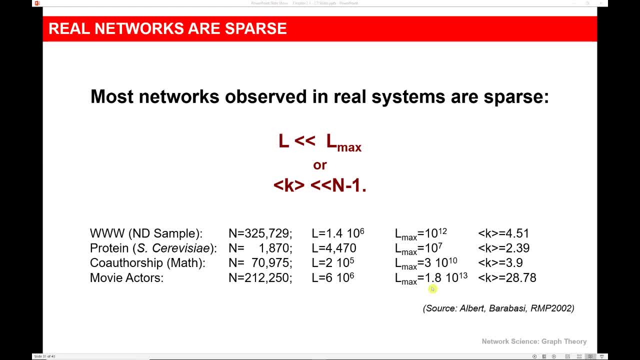 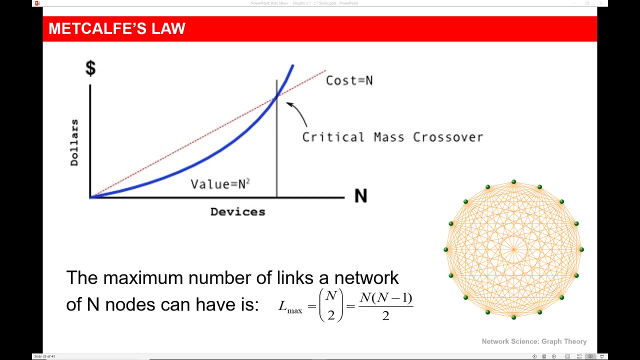 the network had acted in at least one movie with every other actor would be 1.8 times 10 to the power of 13.. So you can see that the number of links is way less than the maximum possible number of links. If you haven't heard of Metcalfe's law, Metcalfe's law states that the value of a network is 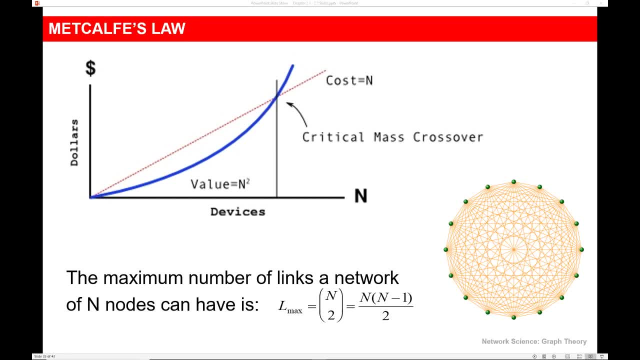 proportional to the square of the number of its nodes. Metcalfe formulated this around 1980. Based on the different networks that communicate, And in the late 1990s this was used as a quantitative valuation for internet companies. So he suggested that the value of a network is based on the square of the number of nodes. 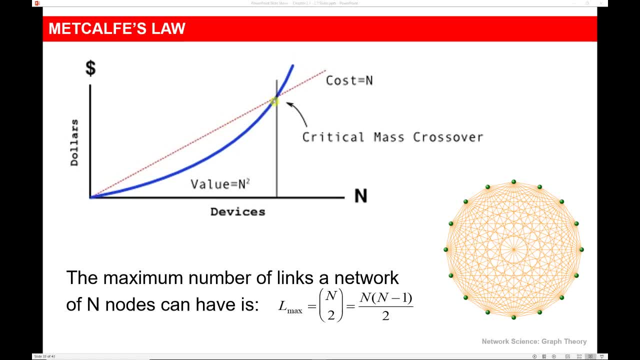 but the cost of using that network was just the number of nodes And the point at which these two values met- the cost and the value of the network. that was where critical mass was reached and the network would start to become profitable. You can think about Mark Zuckerberg making Facebook. 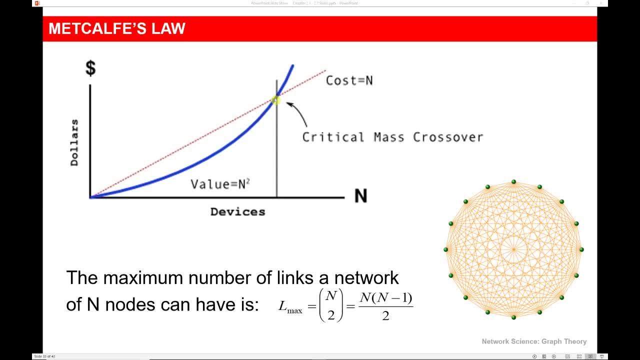 And after he started adding advertising to each page, he would generate more revenue the more people were involved with the social network. The truth is, though, because we know that networks, for the most part, are sparse, the value of the network is not actually going to follow this curve. 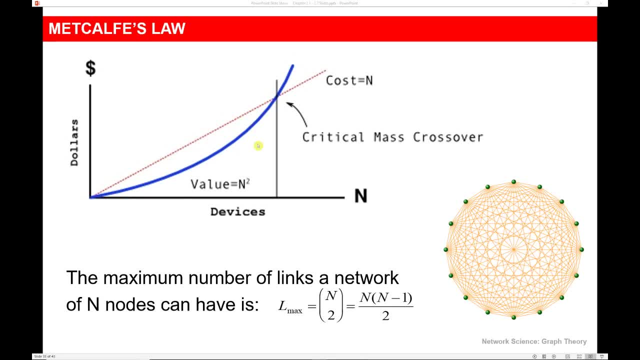 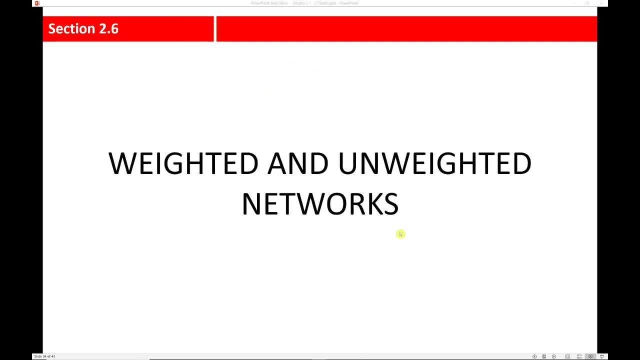 It's going to follow the cost curve. So this is a case where the real world behavior of networks can inform us as to when a network actually becomes valuable Network edges. We also have weights, So we can have both weighted and unweighted networks. 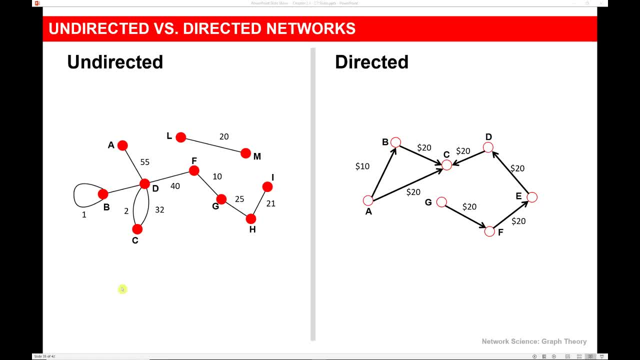 So far we've been looking at networks that are unweighted, So we haven't had any representation of a weight or information that has told us. We haven't had values attached to the different edges in the network. On the left we have an example of a weighted undirected network. 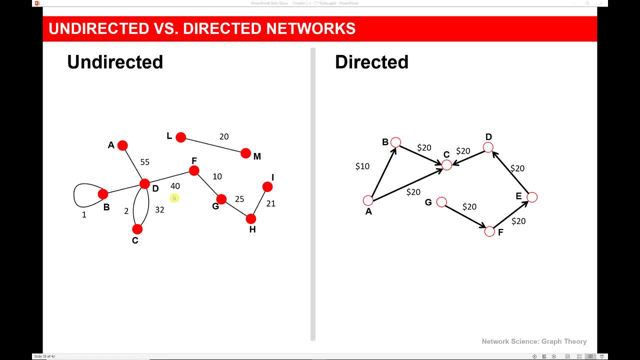 so we haven't had any representation of a weight or information that has told us. We haven't had values attached to the different edges in the network. On the left we have an example of a weighted undirected network. For example, the edge AD has a weight of 55.. What I suggested 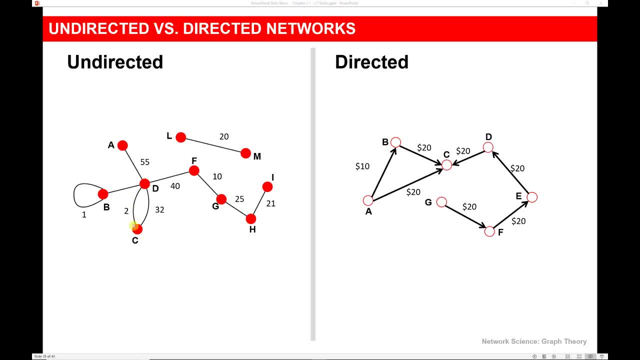 earlier was that in this network we're representing a couple of different relationships between nodes. So perhaps this is a network of how many nodes are in the network and we're representing a couple of different relationships between nodes, So this is a network of how many. 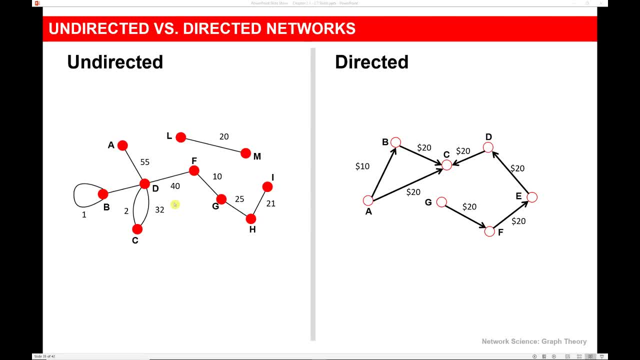 times different people in an organization have had lunch together on company expense, as well as how many times they've had breakfast together on company expense. So we can explain the connection between C and D. Maybe they've had lunch together 32 times on company expense and breakfast twice together and person B has actually treated him or herself. 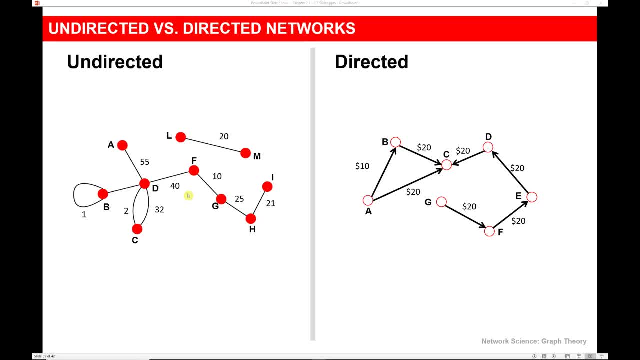 one time. Now the weights do not have to be positive. We can actually have negative weights in a graph as well. So we can actually have negative weights in a graph as well. So we can also have weighted directed networks. This could be a network of how much it costs to deliver. 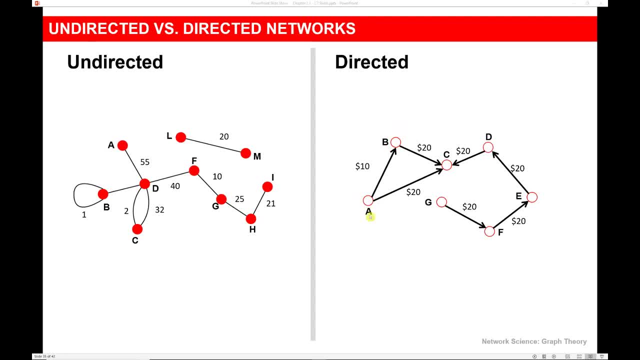 an item from node A to node B and so on. So the majority of these links have $20 as the cost, but delivering from node A to node B is a little bit cheaper. We can also have negative edge weights in a directed graph. Those can actually pose a lot of problems for pathfinding, as we'll. 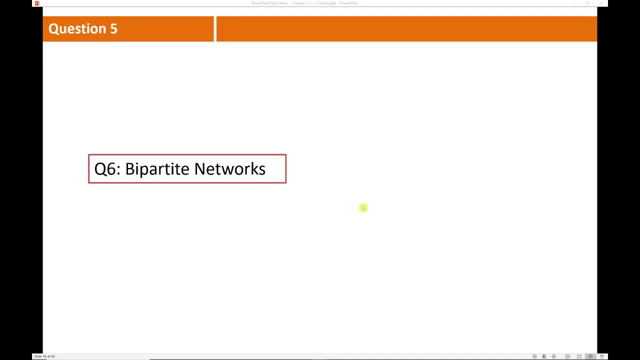 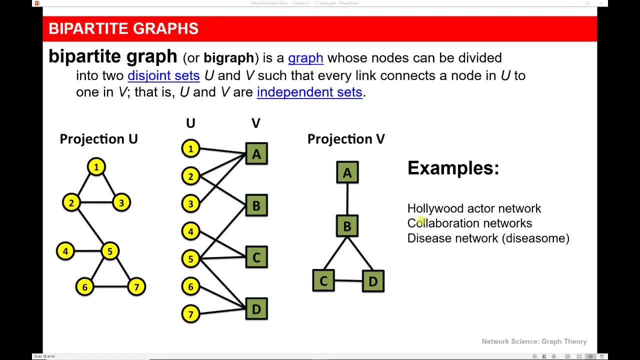 find out later. There's a special type of network called a bipartite network. We'll take a look at here. In a bipartite graph or network we have nodes that can be divided into two sets. So in a bipartite graph we have two separate sets of nodes, where inside one of the sets of nodes there are no. 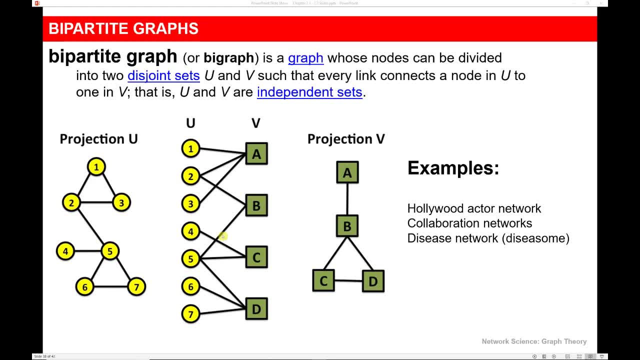 links among those nodes. So let's take the example of different people who are fans of different sports teams. So we'll say that we have seven different people and they are fans of four different sports teams. So person one is a member of a different sports team and person two is a. 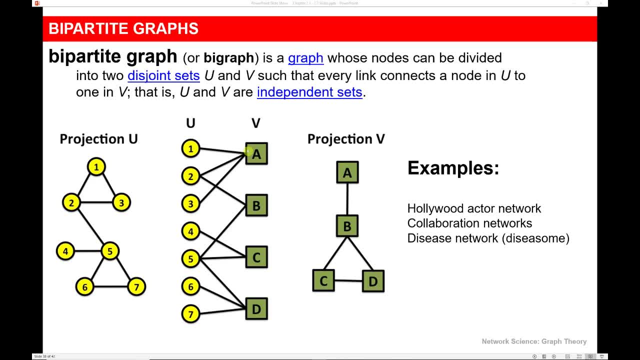 fan of team A, Person two is a fan of both team A and team B, Person three is a fan of team A, and so on. What you notice is that we don't have relationships between fans. We're only representing if a fan is a fan of a specific team. nor do we have any relationships among teams. 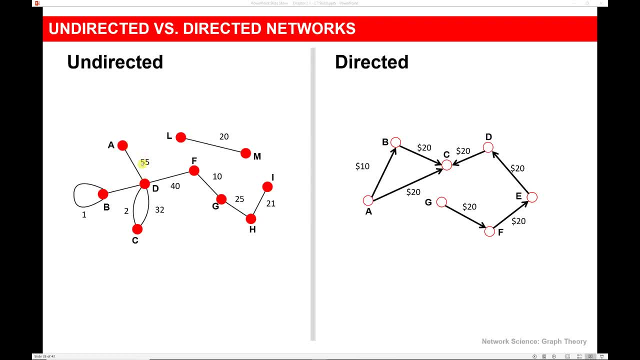 For example, the edge AD has a weight of 55.. What I suggested earlier was that in this network We're representing a couple of different relationships between nodes. So perhaps this is a network of how many times different people in an organization have had. 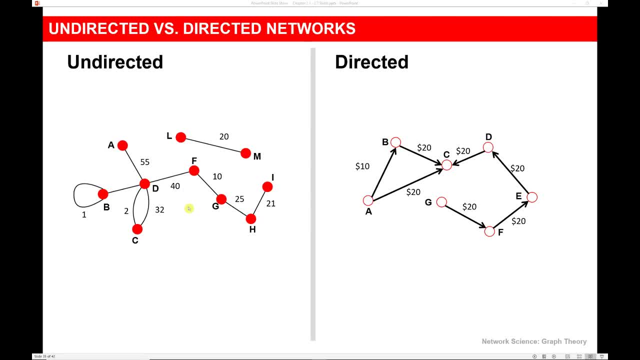 lunch together on company expense, as well as how many times they've had breakfast together on company expense. So we can explain the connection between C and D. Maybe they've had lunch together 32 times on company expense and breakfast twice together. Person B. 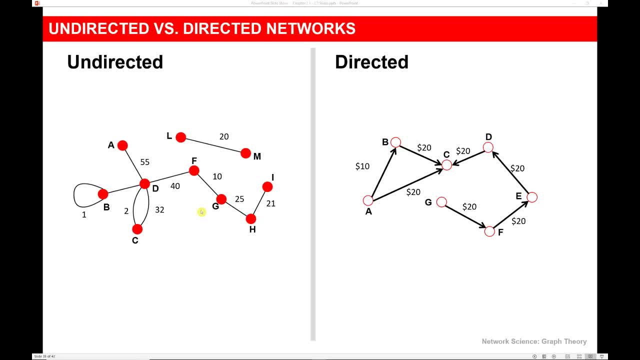 Actually treated him or herself one time. Now the weights do not have to be positive. We can actually have negative weights in a graph as well. We can also have weighted directed networks. This could be a network of how much it costs to deliver an item from node A to node B, and 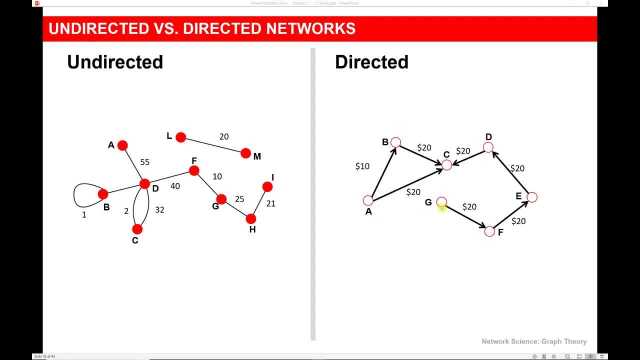 so on. So the majority of these links have $20 as the cost, but delivering from node A to node B is a little bit cheaper. We can also have negative edge weights in a directed graph. Those can actually. There's a lot of problems for pathfinding, as we'll find out later. 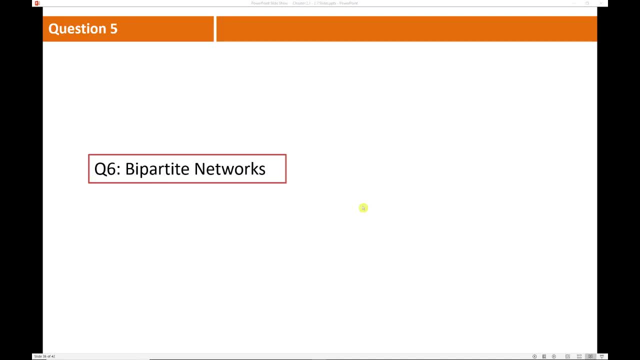 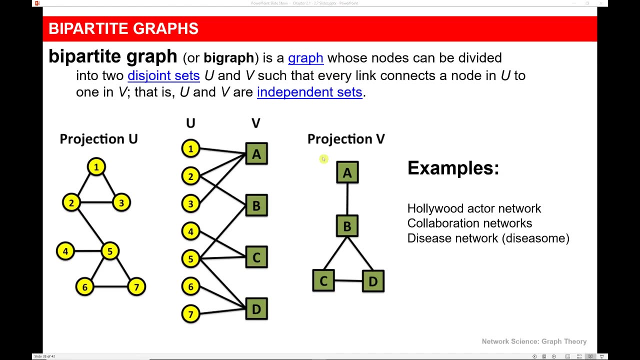 There's a special type of network called a bipartite network. We'll take a look at an example here. in a bipartite graph or network We have nodes that can be divided into two sets. So in a bipartite graph we have two separate sets of nodes, where inside one of the sets 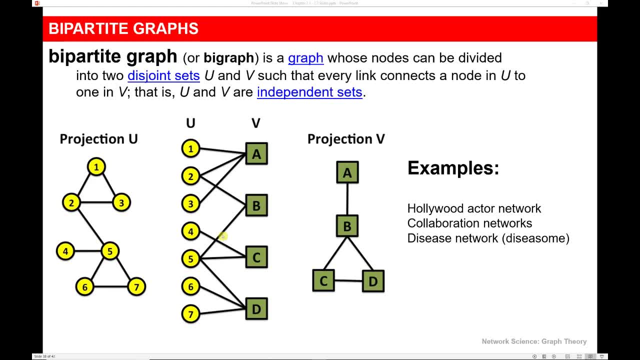 of nodes. there are no links among those nodes. So let's take the example of different people Who are fans of different sports teams. So we'll say that we have seven different people and they are fans of four different sports teams. So person one is a fan of team a. person two is a fan of both team a and team B person. 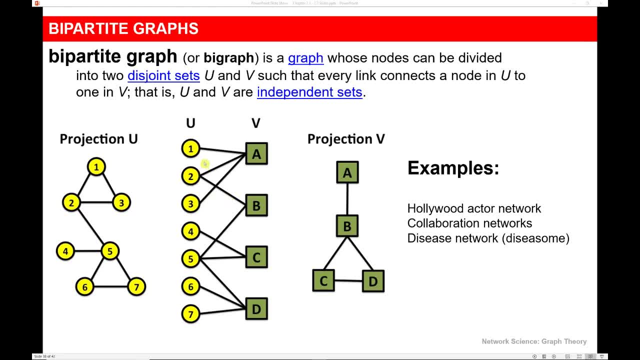 three is a fan of team a and so on. What you notice is that we don't have relationships between fans. We're only representing if a fan is a fan of a specific team. nor do we have any relationships among teams. So in a case like this, we have what's called 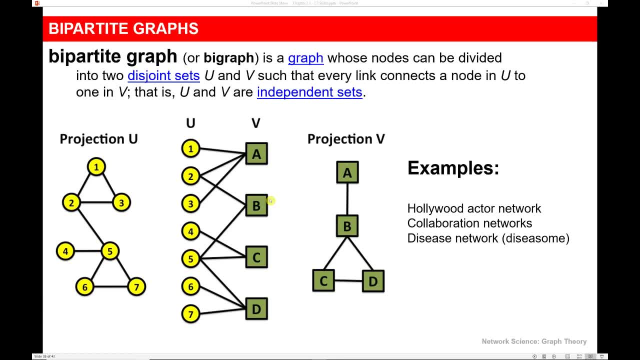 A bipartite graph and we can create what's called a projection for each set in the graph. So we can actually create a graph of the fans as well as a graph of the teams based on how they're connected, And we can do this automatically using the tools that we have.